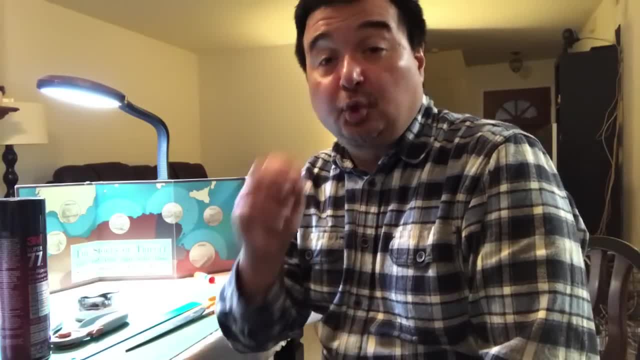 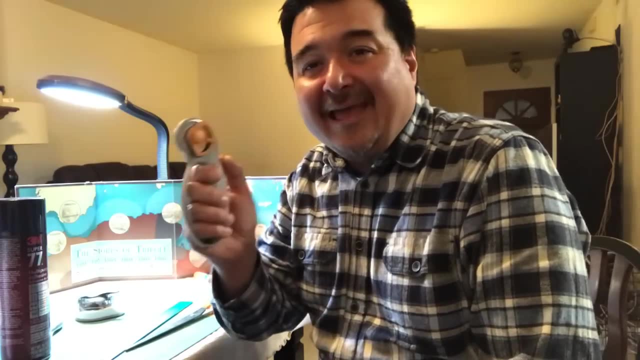 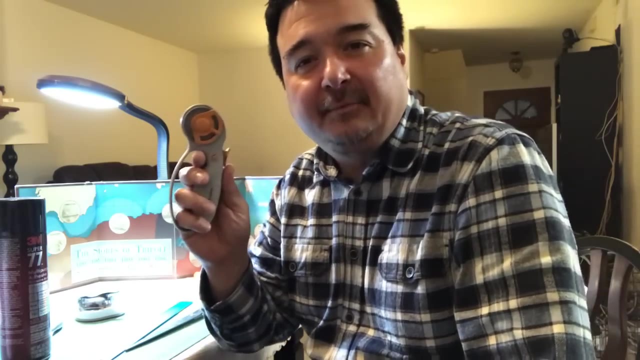 cards. For now, let's go over the tools and items that we are going to need for this build. So I use a rotary cutter. this is a Fiskars rotary cutter. I've had this for many months and this is going to be the primary implement that I use to cut. 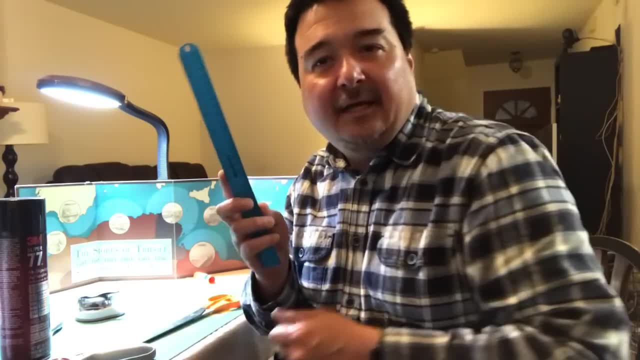 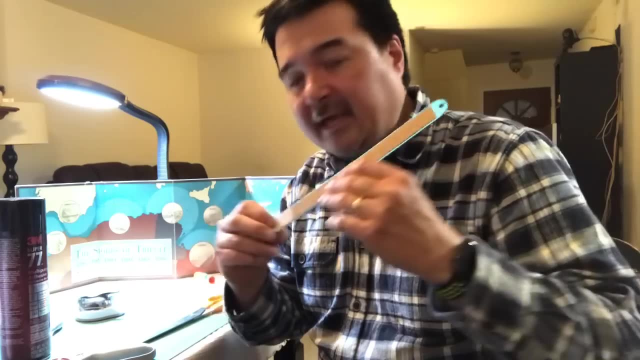 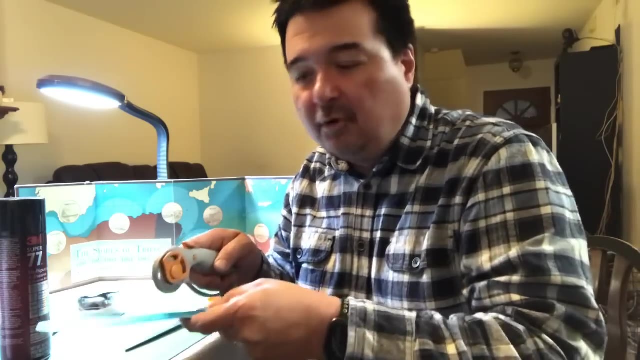 out the cards from the paper And you need a nice straight edge ruler. I have a nice metal back ruler, or rather a metal ruler with cork backing, and the cork backing, or rubber backing, is important so that when you are cutting the ruler doesn't slide or move, it just. 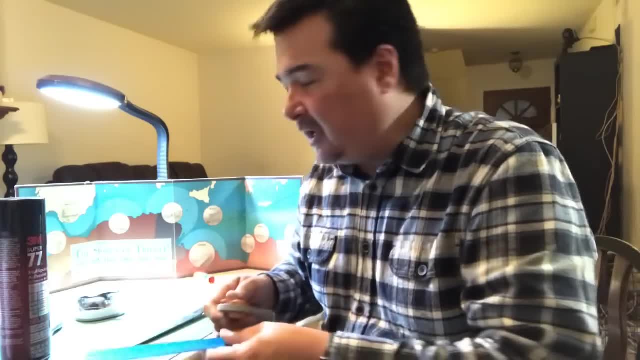 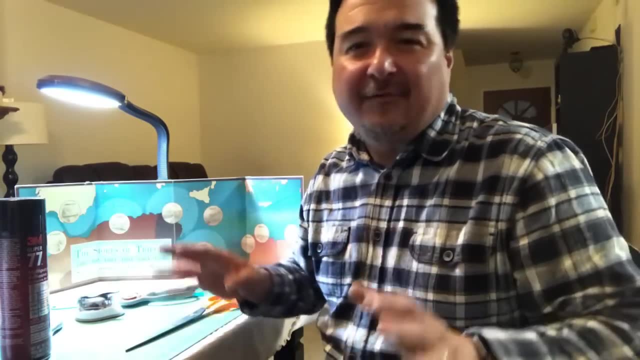 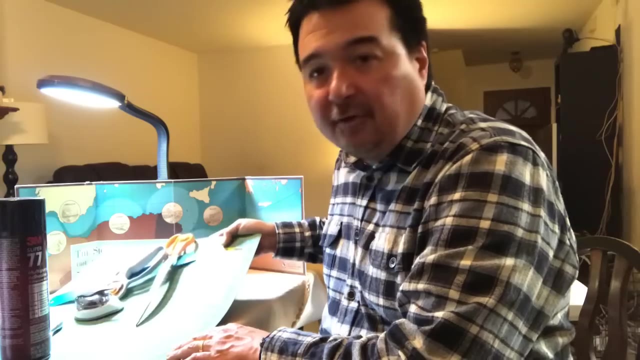 keeps your cutting edge straight on the paper. Now, it won't do too well if you're cutting directly on your table. you don't want to damage anything around the house when you're making a print and play game. So I have a self healing mat, and this is a brand called Olfa. you probably can't see it on the video because of the glare. 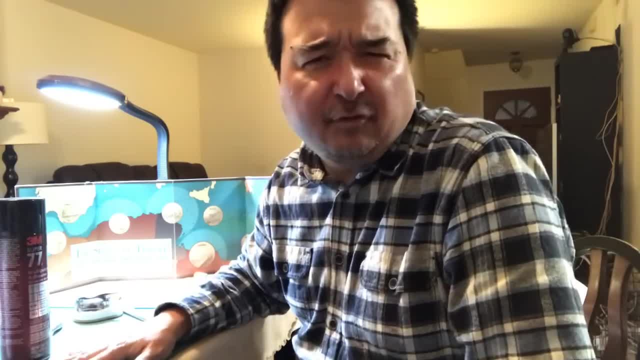 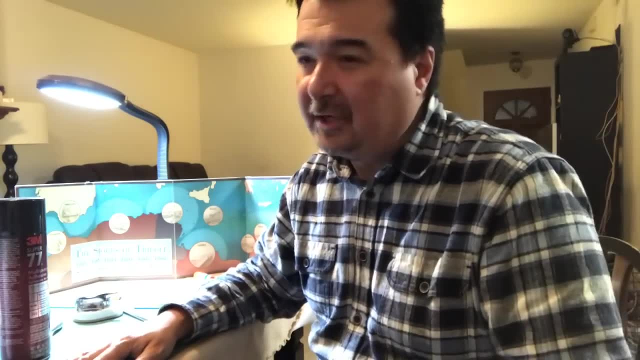 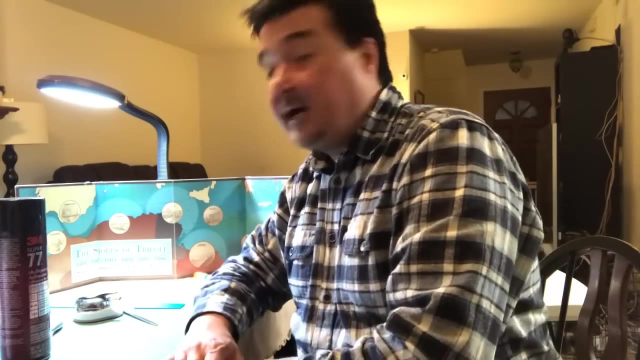 This is an Olfa self healing mat. I've had this again for about eight or nine months. I was fortunate enough to actually find this mat at the thrift store for less than two dollars and it is a very nice big mat. It is about 24 inches by 24 inches or 24 by 36, something like that. 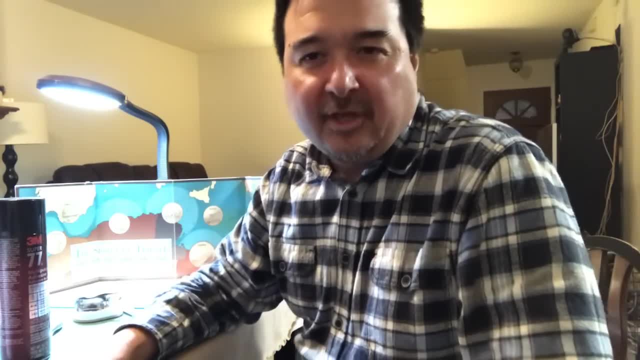 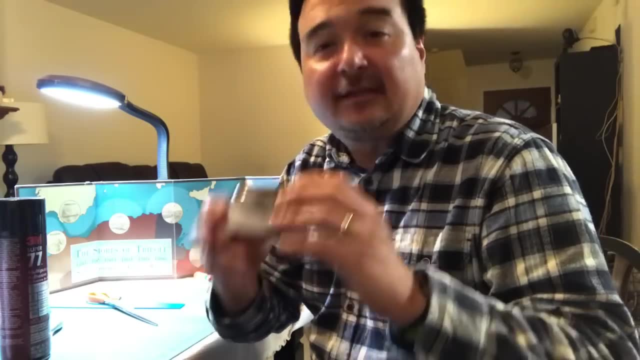 And it does well. You want to be able to round the card corners, and I am gonna use tonight something called the Kadu Maro Pro Corner Rounder. This is- I'll talk a little bit more about this corner rounder, and I've also made a video specifically on this in the past. 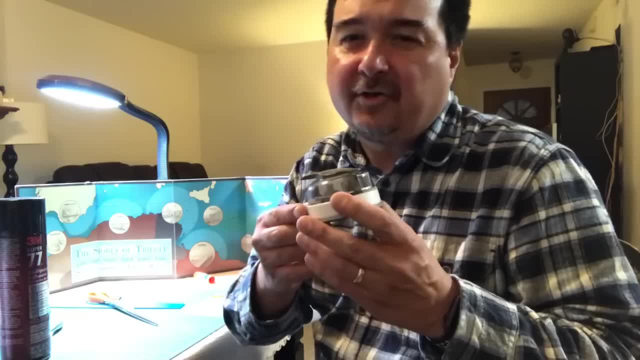 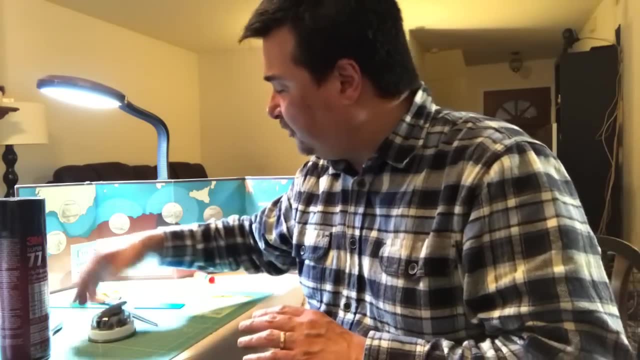 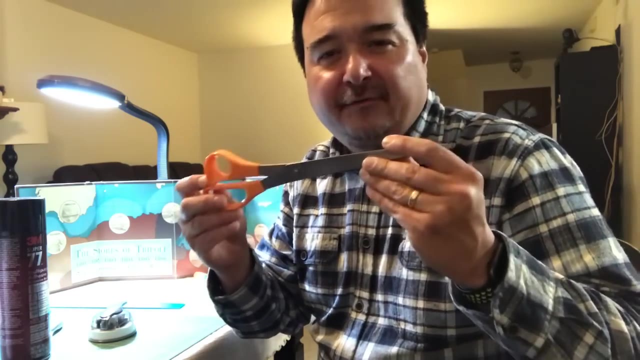 But I really like this guy. it's less than $10. I bought it on Amazon And I've used it on many, many builds And this gives you nice rounded card corners. I will also be probably- I don't know- if I'll need a pair of scissors, but I like to have a nice heavy-duty pair of scissors handy. 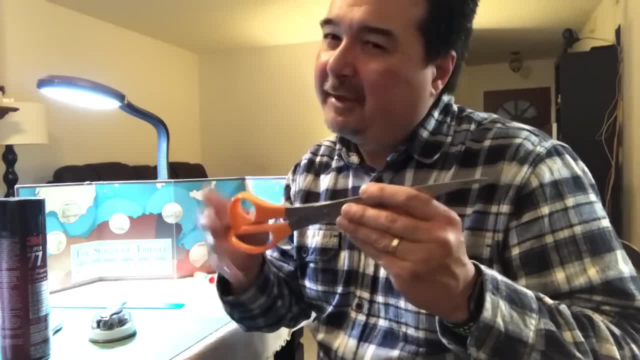 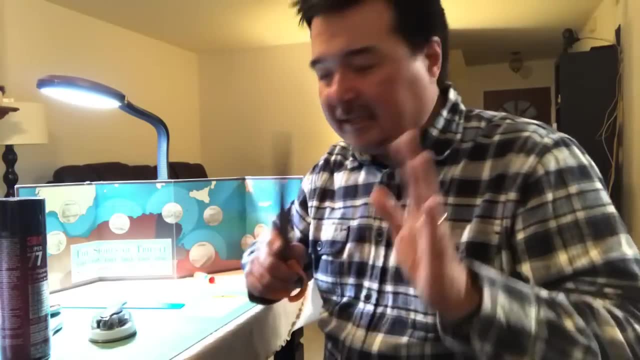 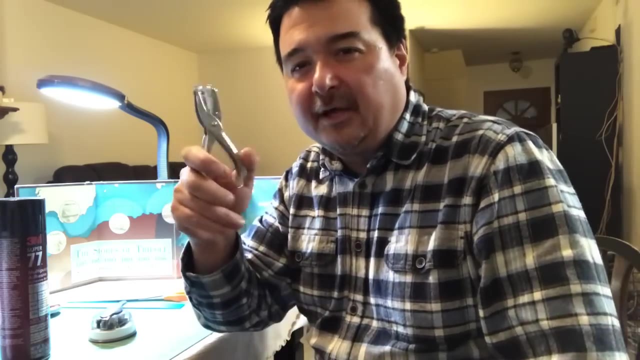 This is Fiskars brand scissors. You're probably starting to see that I like the Fiskars brand. My scissors are Fiskars brand, My rotary cutter is Fiskars brand and I like those things. One final piece that I like to use to align my cards is a hole punch, just a single hole punch. 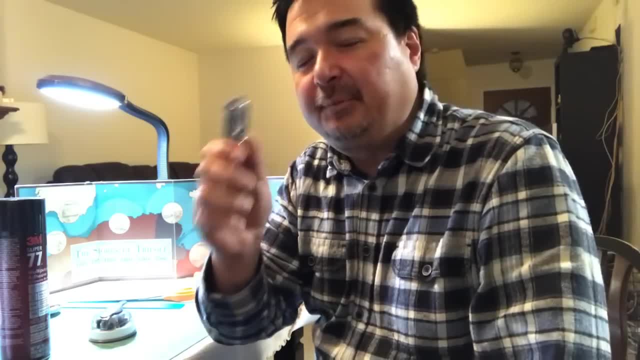 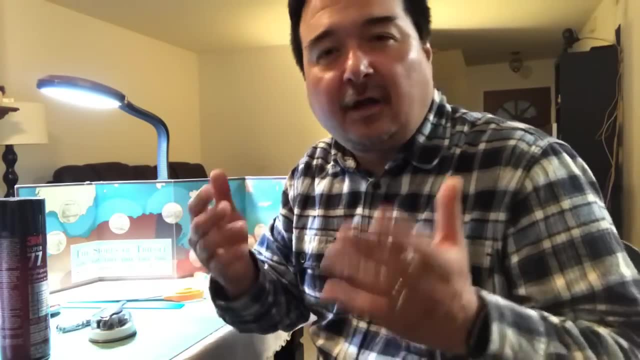 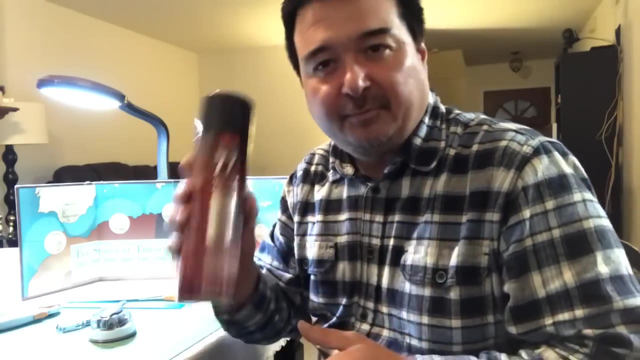 here and I will attempt to show you exactly how this comes into play when I am aligning the fronts and the backs of my cards a little later on. How are we going to adhere the cards, the three layers of paper? I use 3M Super 77 spray glue for that purpose. This is a can that's already I've used. 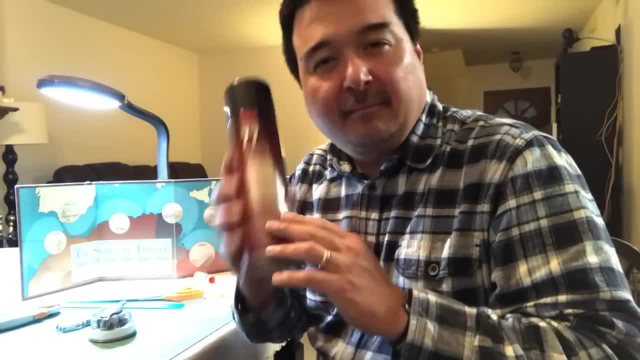 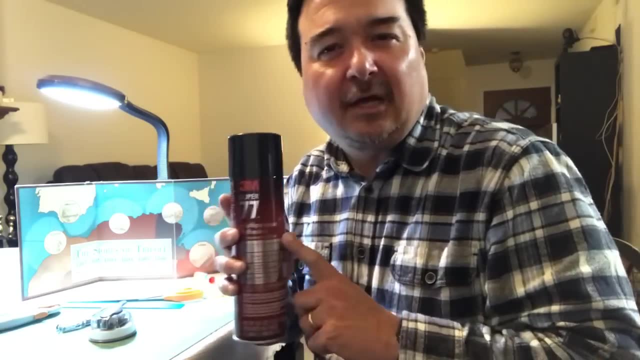 it for three or four builds already and it's running low, but I think it should be just enough for the task that we have to do tonight. This can is about $10 from the Home Depot and it lasts me for three or four or even five builds. 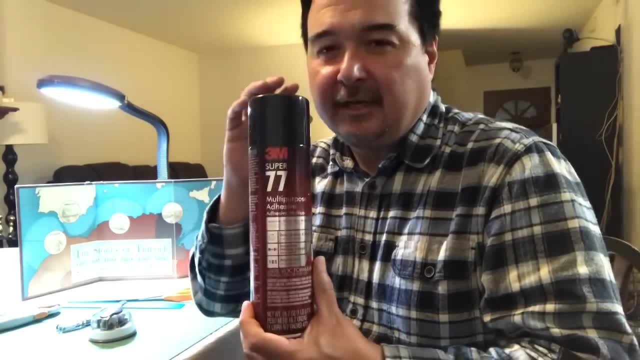 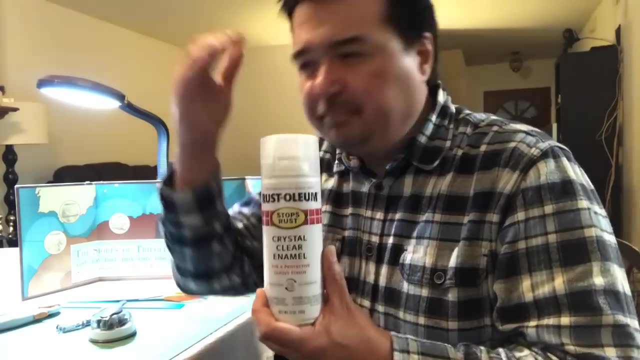 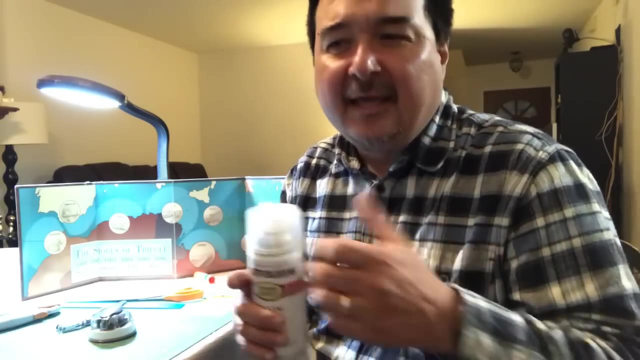 Sometimes, and this is my favorite brand of spray glue to use for making cards. Finally, I like to have a put a, put a gloss, a coating of clear gloss enamel on the cards, both to seal the ink and to give the colors a nice bit of pop. and another thing is it tends 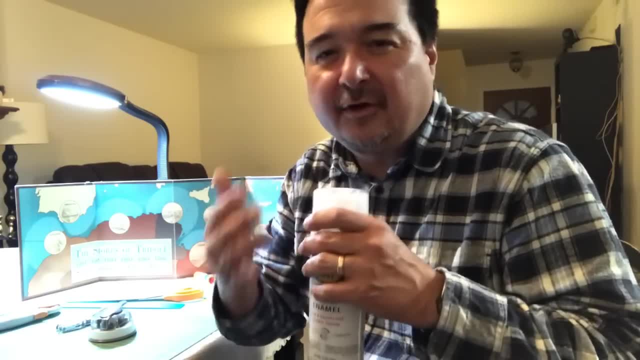 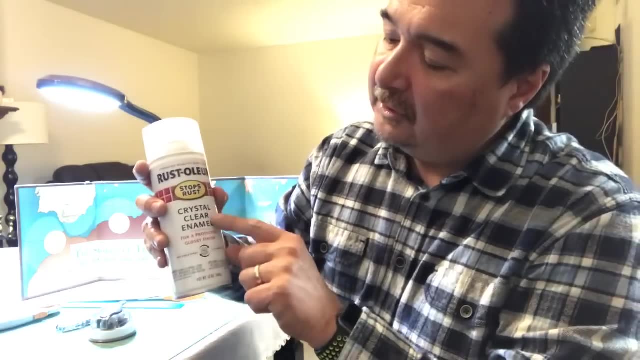 to make the cards a little bit more smooth and slide against each other, maybe lessen the friction of the paper against each other. For that purpose I currently use Rust-Oleum Crystal Clear Enamel®. you have to make sure you're getting the clear. 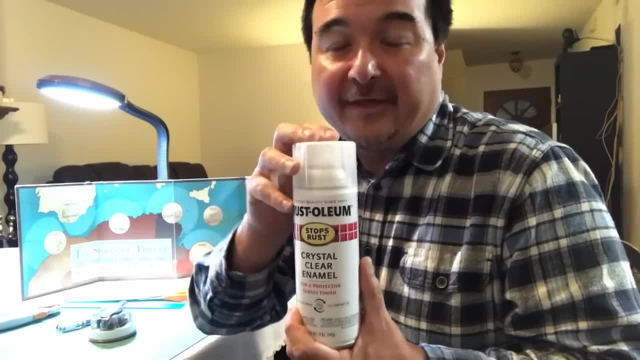 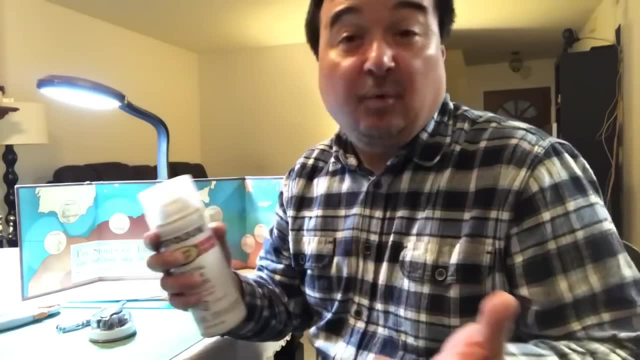 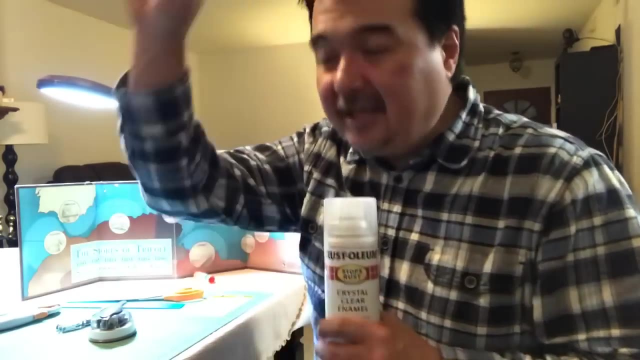 one. I made the mistake before of getting one that was not clear and it was actually colored almost like spray paint. Then, when I sprayed on the card sheet, I was very surprised, rudely surprised, to see that a nice white sheen- unremovable and permanent- had covered up the 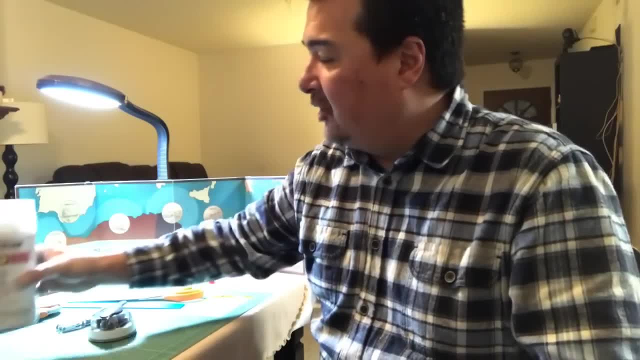 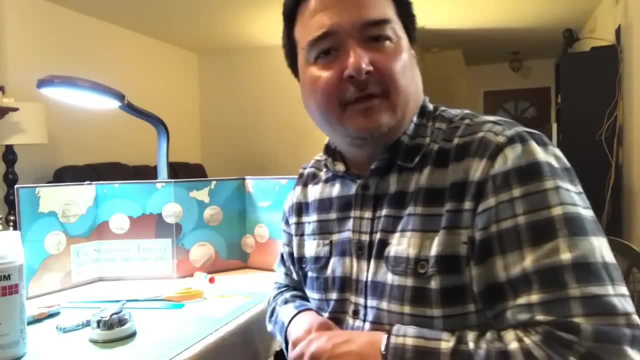 cards, and I had to redo that, the clear one. All right, So those are our main tools and supplies that we're going to be using. Of course, you're going to be using some paper as well in my printer, So let's get things together. 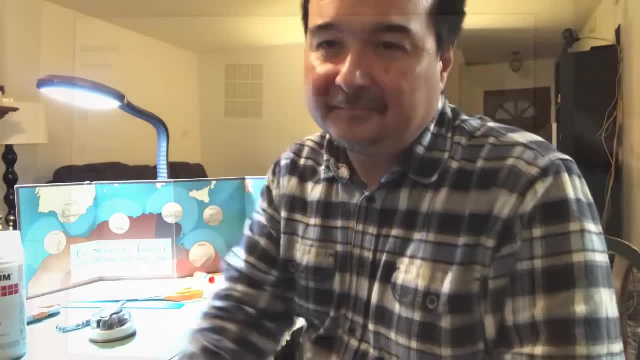 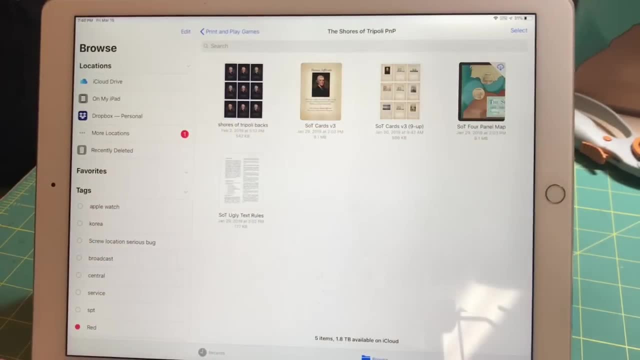 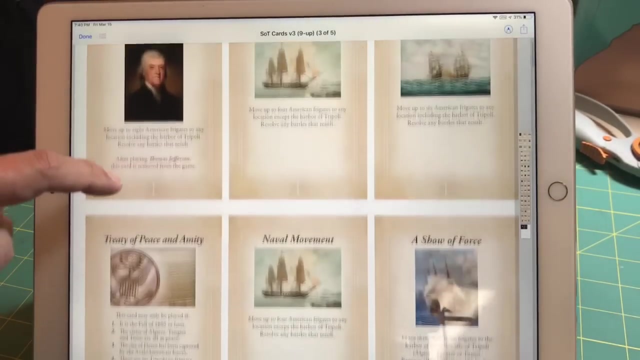 I'll see you at the table and let's make some cards Right. The first step is we have to print out the card files. So these are the card files that I got from Kevin. I've got them loaded up on my iPad and we'll take a look at the card fronts here. So these are the card fronts for the game. 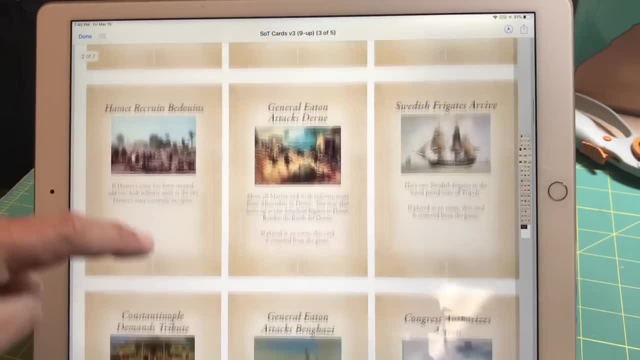 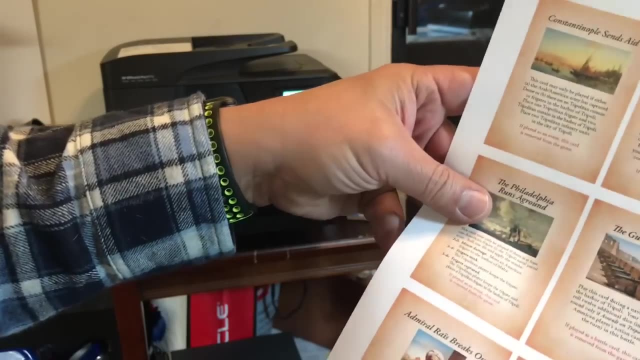 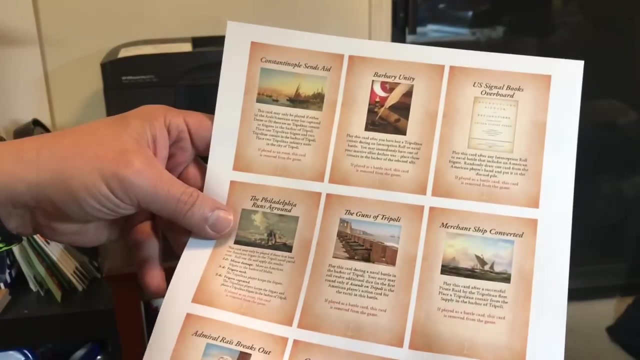 Shores of Tripoli And there are seven pages of cards to print out here. Here you go. So that's what my printout looks like, And you know, we're going to go ahead and make five more of these pages and then we'll print the card backs and then we'll move on to the next step of the process. 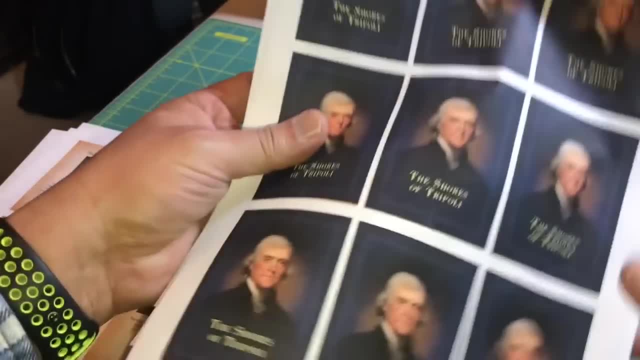 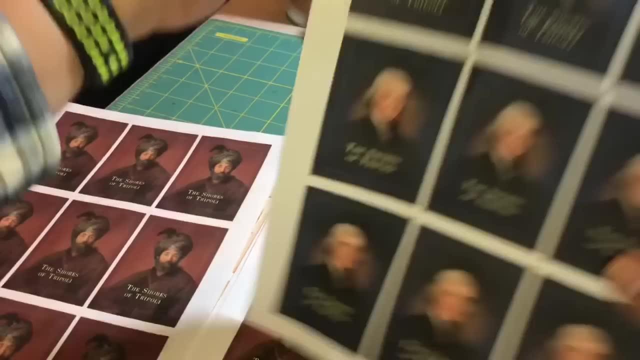 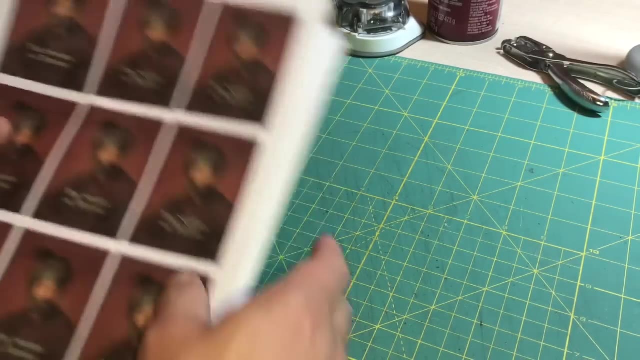 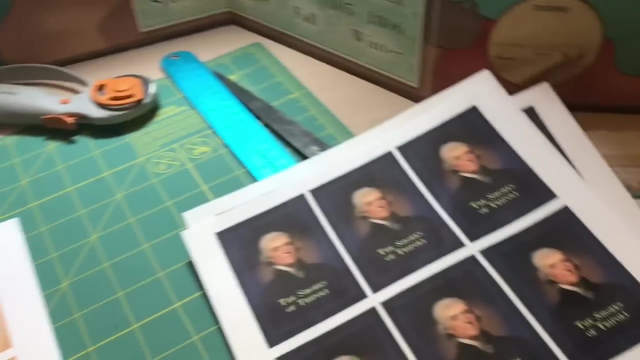 So here is the US card back and I'm going to move it to the US side Tripolitan card back until we have three copies on each side. Right Now we have the complete set of card fronts and backs for the Tripolitan side as well. We have the complete set of fronts and backs for the US side. 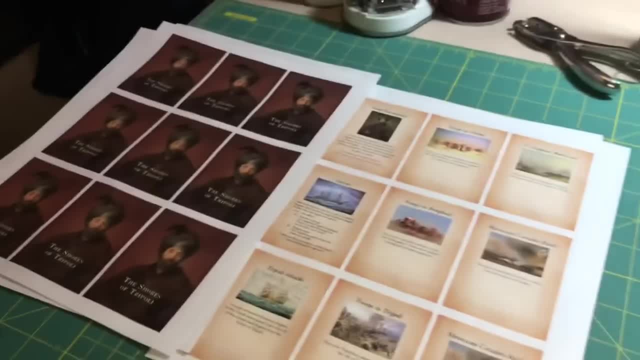 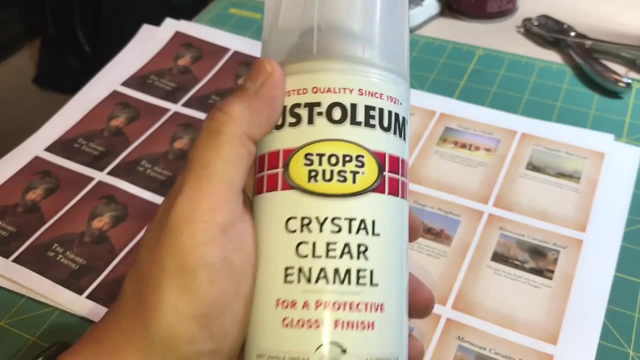 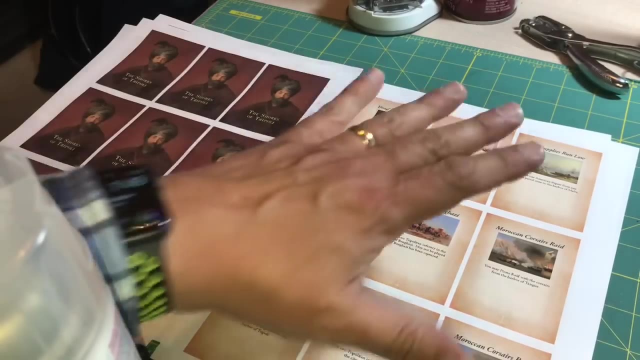 Now, that's step one. Step two is we are going to treat these cards with the Rust-Oleum enamel, And once again, the purpose of treating them with this is to seal the ink so that it doesn't smudge or smear and to give the cards a nice glossy finish and also to kind of like make the. I find 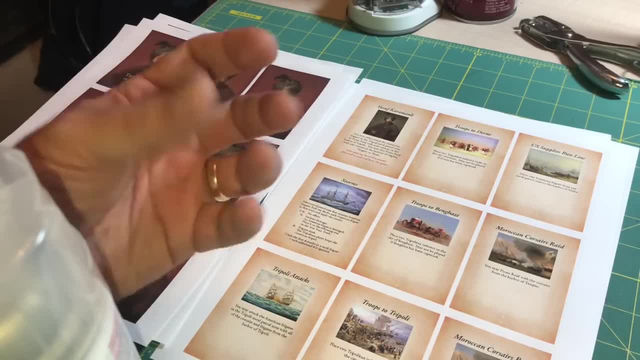 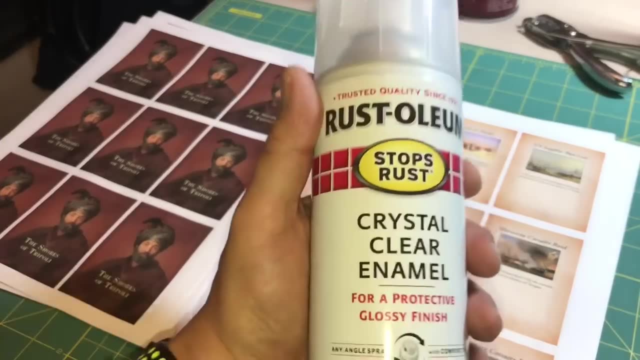 that it makes, for me at least, it makes the colors of the of the printout pop and look extra vibrant. I would love to show you this, but I'm going to have to do it outside the house because this stuff doesn't- I mean, it tends to stink. 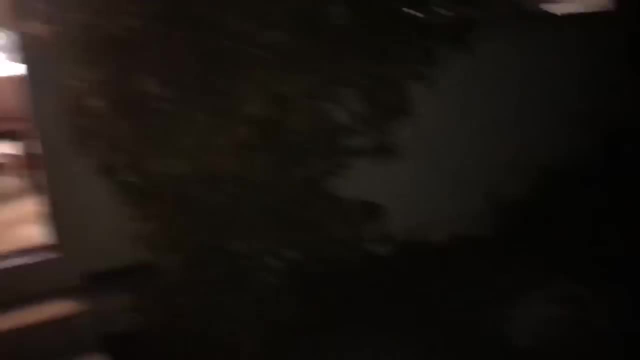 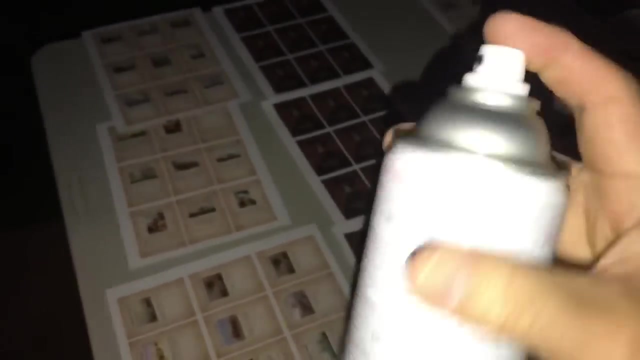 up the entire house. I'm not going to spray it in my office. I am outside my house, There is my house over there and I'm in the backyard and here is my can- Rust-Oleum and I'm going to go ahead and spray these cards. 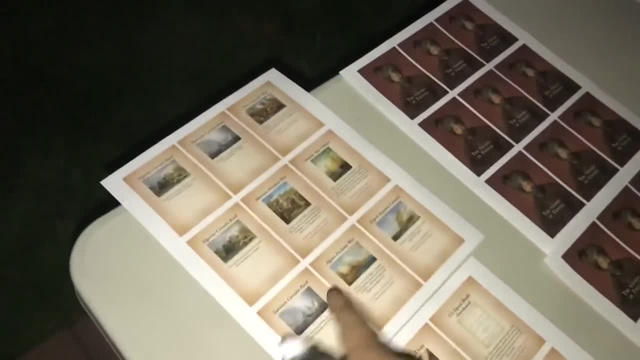 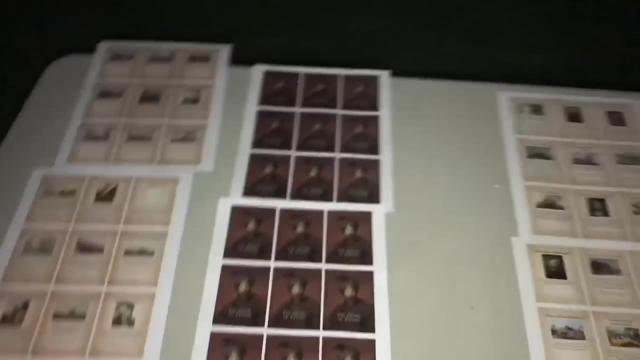 You really don't need to spray a lot, because a little goes a long way, And I really don't. Ok, make these cards super soggy, okay, so that's about enough, and we're going to let all that stuff dry for about 15 to 20 minutes and then we'll move on to the rest of the process. 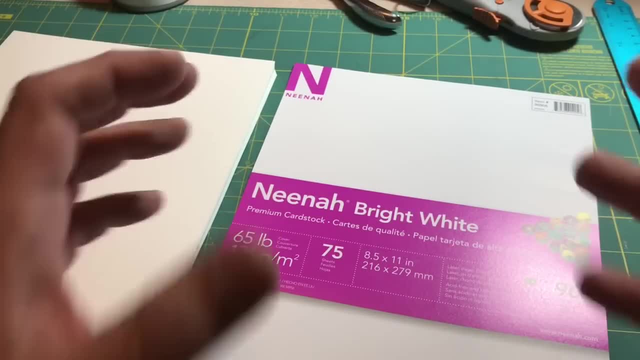 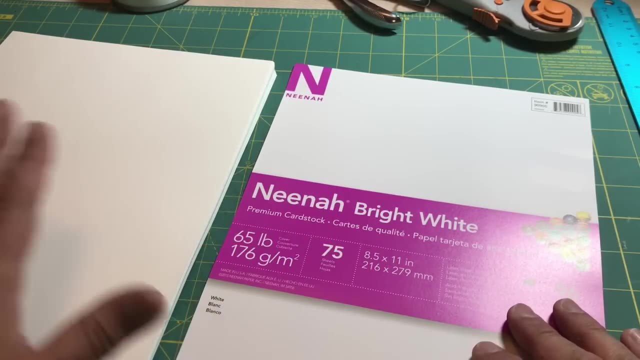 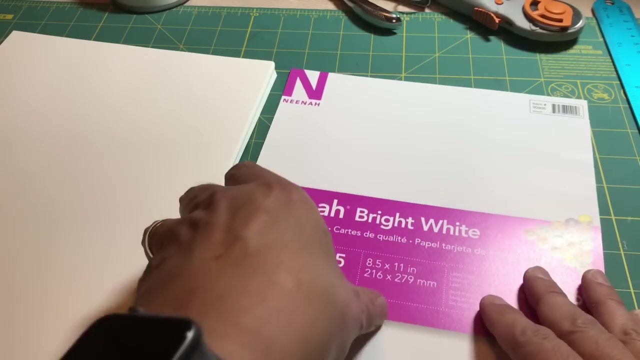 right. while we're waiting for our front and back image sheets to dry from the crystal clear gloss enamel, let's focus on the cardstock that we're going to be using as the layer in the middle between the two sheets of plain paper. so this is the cardstock that i'm using today. this is uh. 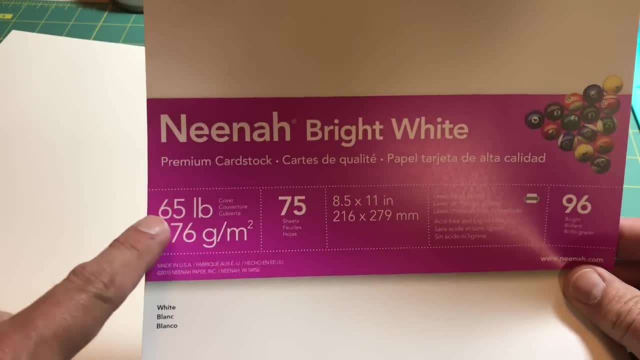 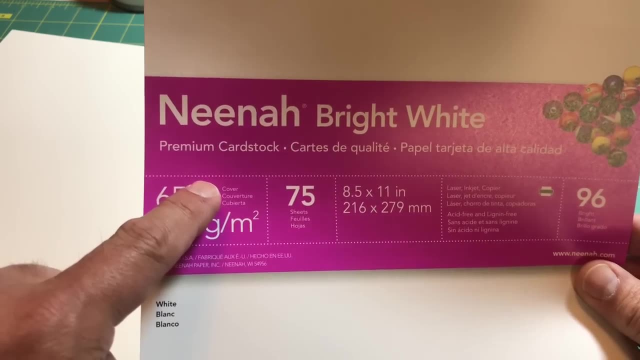 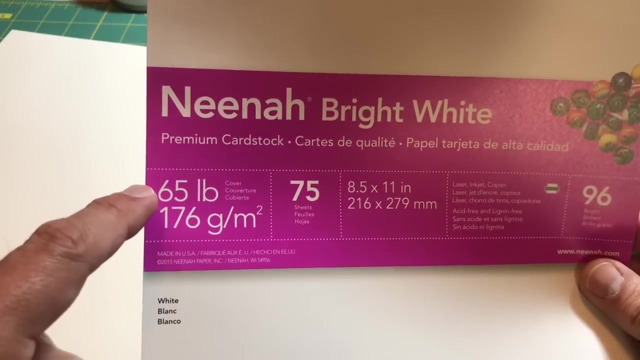 called nina bright white. the uh weight of this cardstock is 65 pounds and that is uh expressed in cover uh sheet that here in the us. what i learned is that there's two um measurements for paper. thin paper is uh measured in like a thinner uh weight uh also in pounds um, but it's a different term. 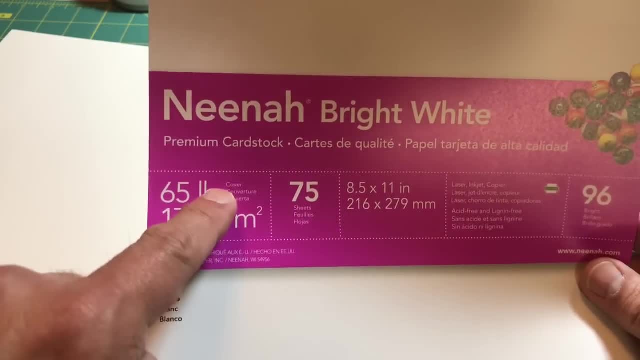 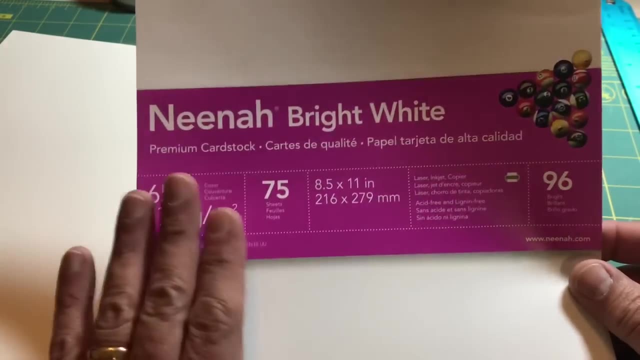 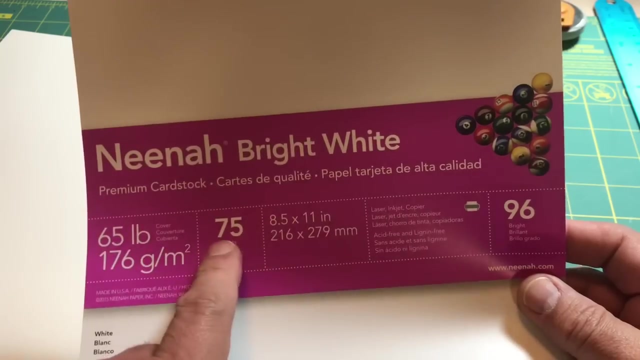 i believe it's called paper weight, and then, uh, thicker paper is measured in what's called cover weight. so this is 65 pounds. so this is a little thinner than i'm usually used to. uh, usually i'll use 110 pound paper, so double the thickness. um, i got this one at target uh for about five dollars. okay, here is 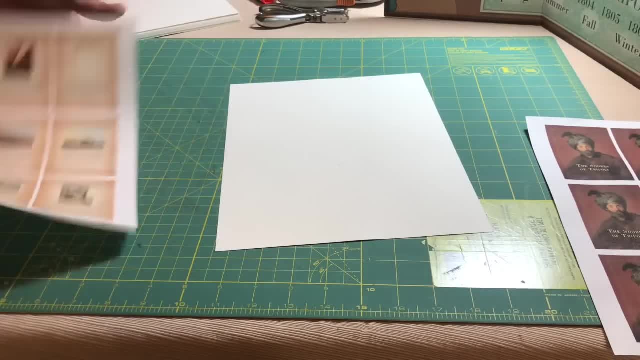 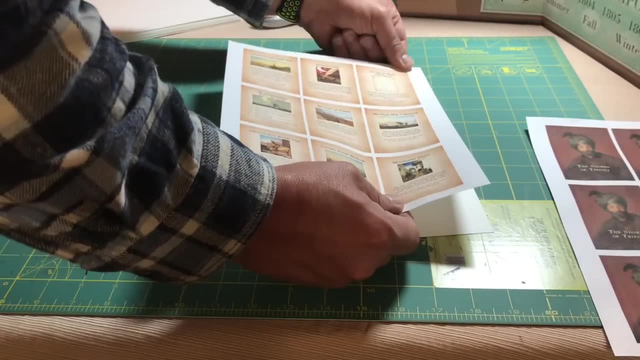 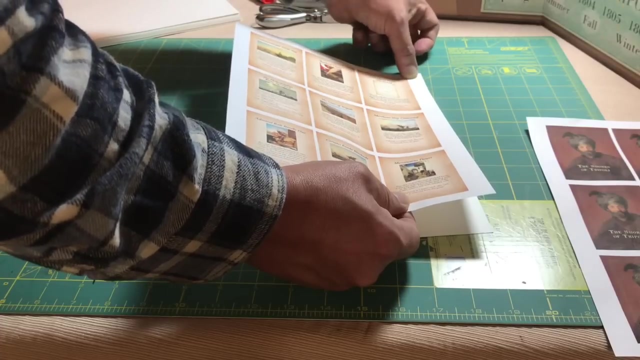 our sheet of cardstock and this already has spray glue on it, and here are our card fronts, and what i'm going to do is i'm going to carefully align the cardstock with the paper and i'm going to cut the card front to one corner, here coming down very precisely, and now one corner is adhered and 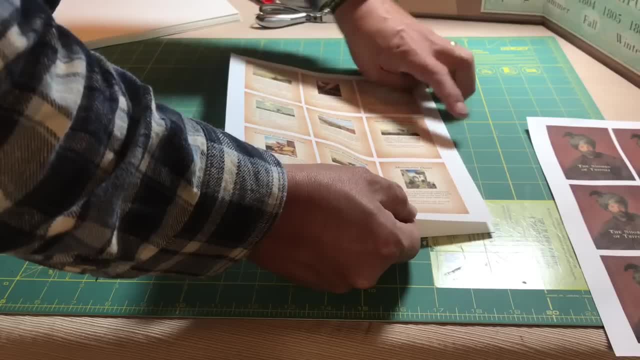 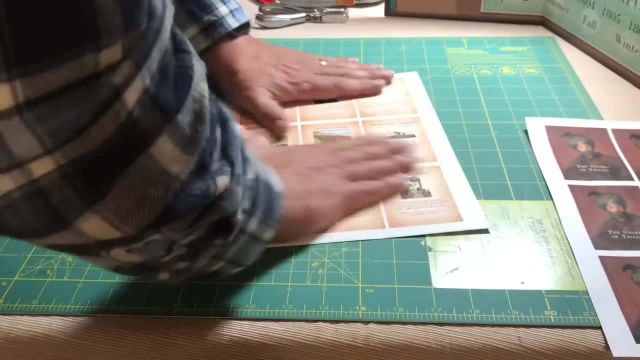 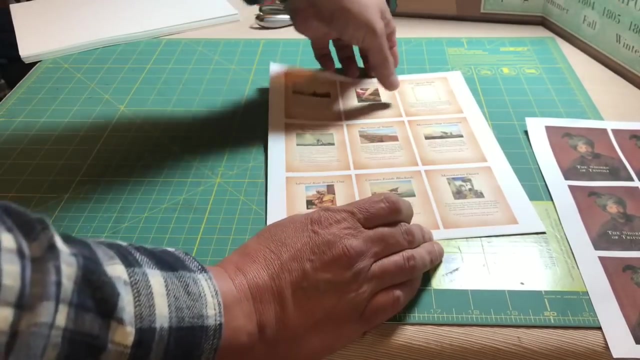 as straight as i can make it, and then i'm going to go ahead and do the same thing for this side over here. essentially, you want these two sheets to be as straight as possible, all right, so that is the card front, and it is now attached to the cardstock. now what we're going to do is we're going to 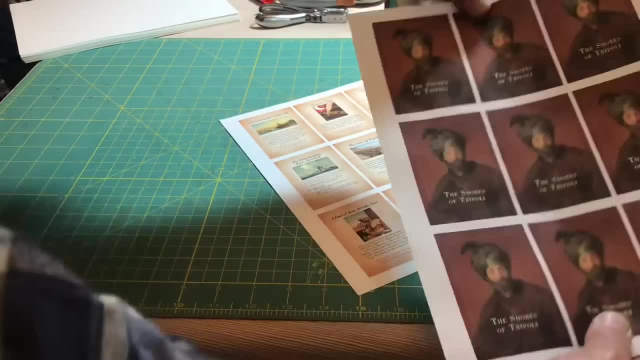 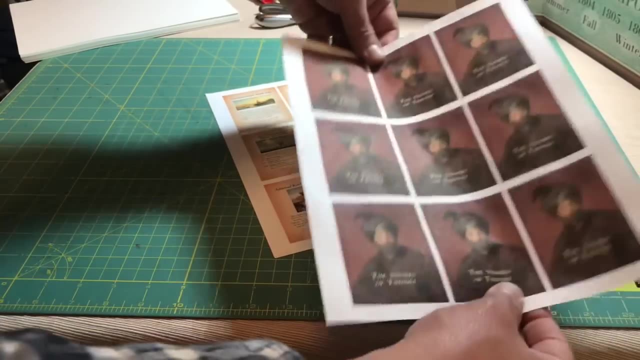 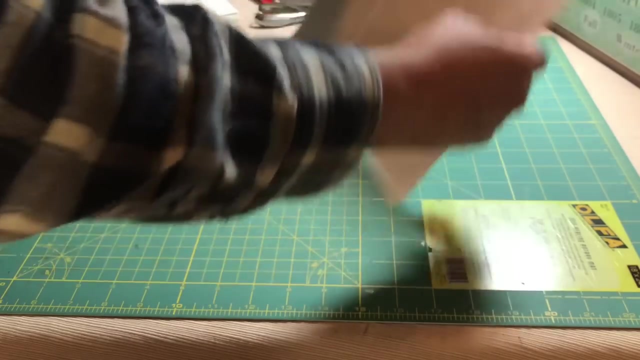 um, we're going to align the card backs to the front so that when we finally glue the backs to the front, they are as straight as we can make them. and here's how that's going to happen. i am going to lay the backs on top of the fronts, like so, and then i'm going to use this light i just want to make. 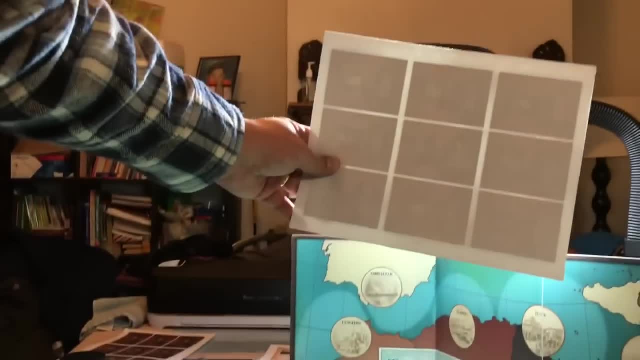 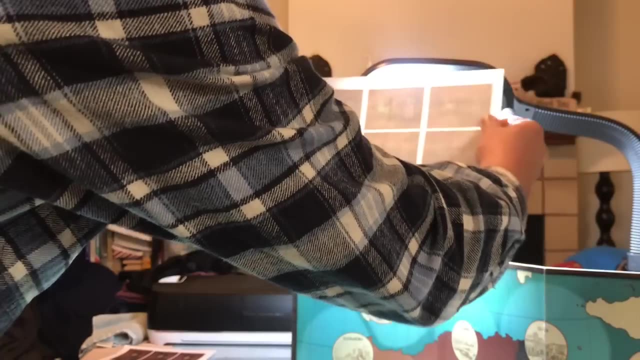 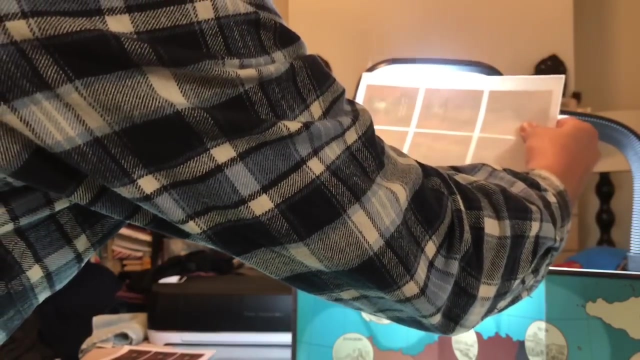 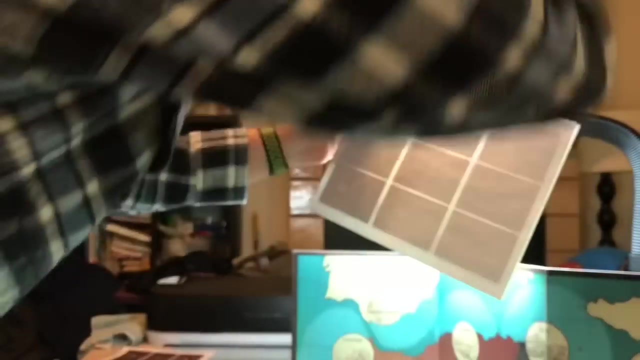 sure that you can see what i'm doing here, and i'm going to use the light to align the card fronts and the backs as much as i can, as best i can, until i only see one image. the front and the back are basically merged, and once they are merged i will then make a note of that, that alignment using the 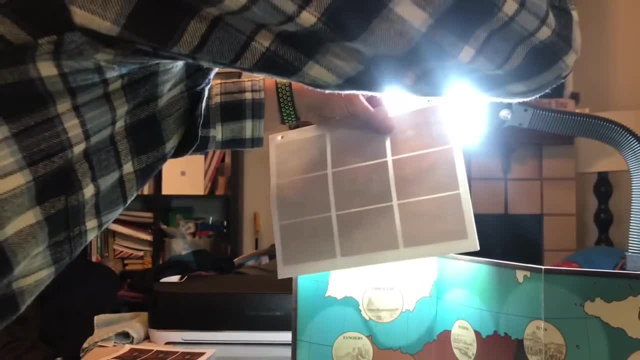 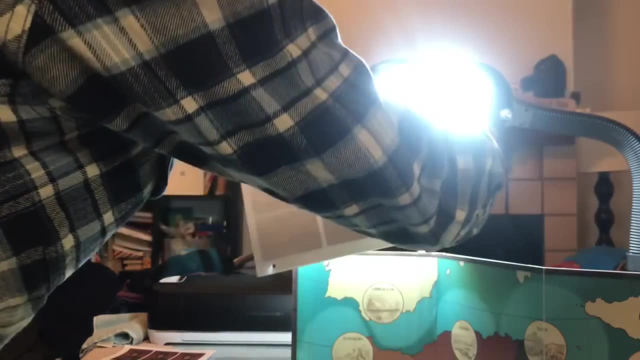 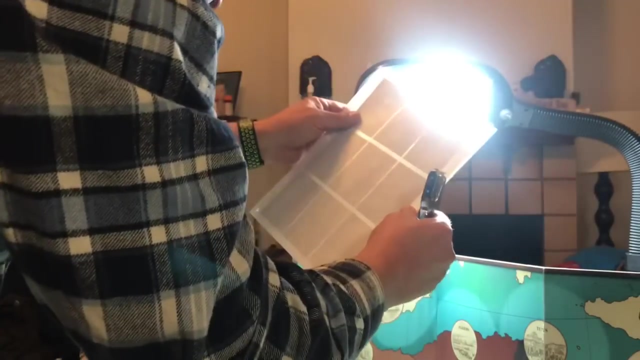 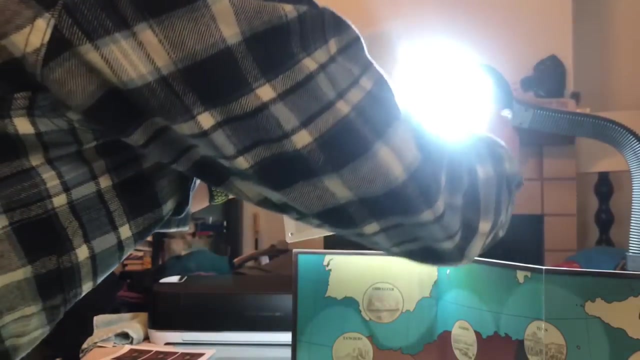 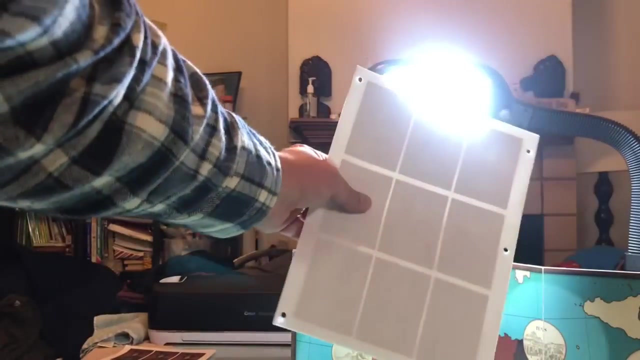 single hole punch. okay, a little bit of glue, and then i'm going to go ahead and glue the card back and i'm going to go ahead and glue the card back. so the idea here is, when i finally go to glue the card backs, i line up the holes and i should get a pretty good front back card alignment. 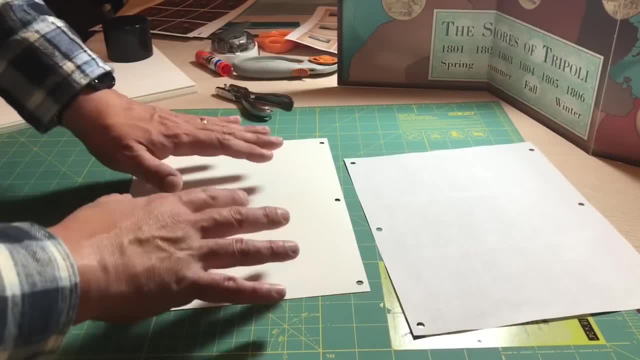 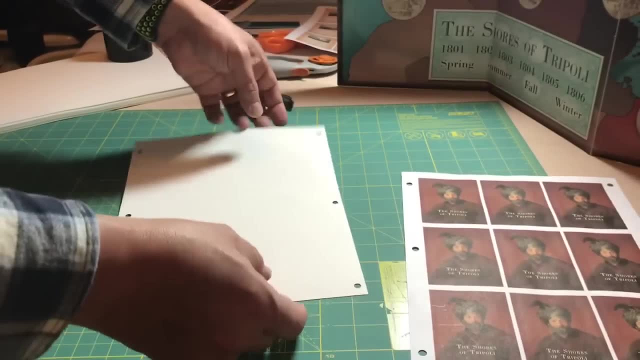 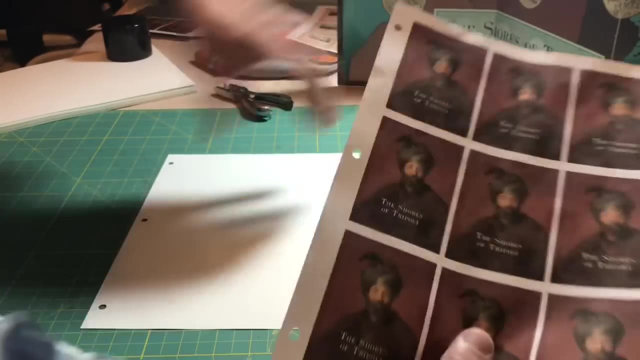 using my craft lamp over here, so i hope you guys saw that and i hope that that explanation made sense. here are the card backs and of course, you want to make sure that this is properly aligned. here's the top and this is the top of the card backs. i have definitely had it happen where i aligned. 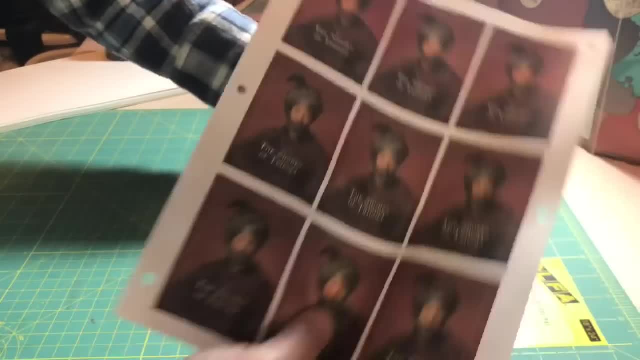 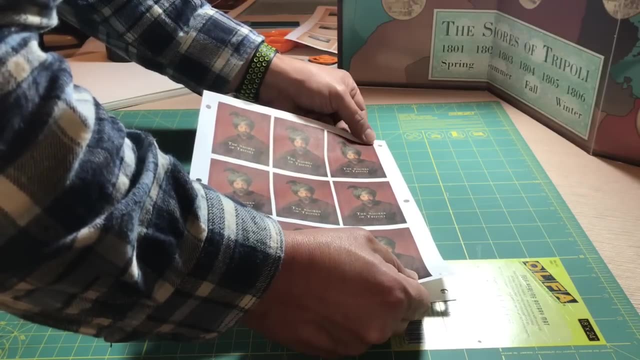 things. i, i didn't, i failed to check and then i uh, did misoriented things and then i had to do stuff over. so now what we're going to do, because we had made those holes earlier, we are now going to align the backs so that the holes are as 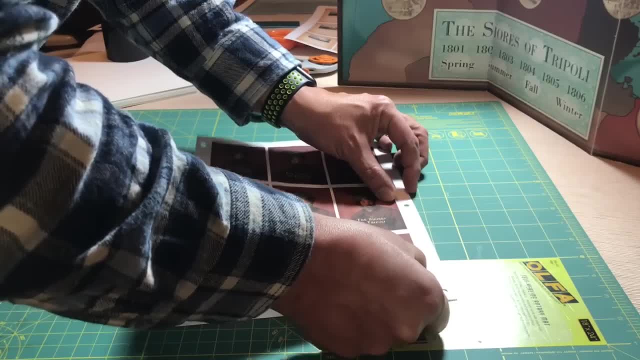 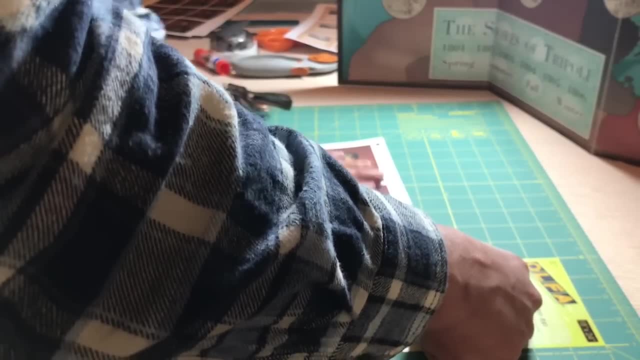 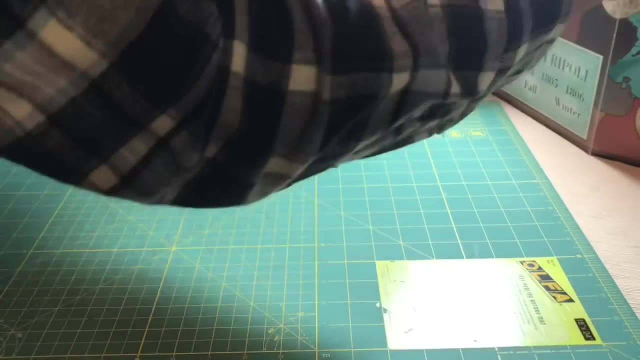 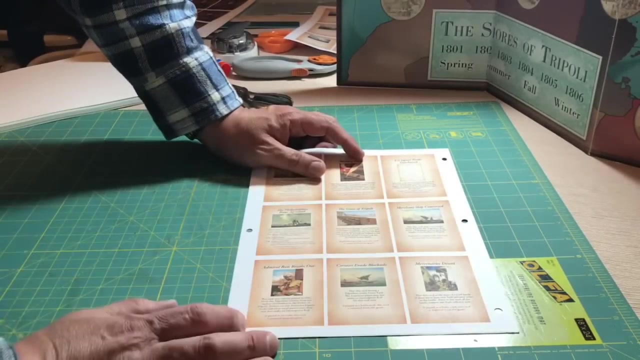 straight, as straight as we can make them. so there you go. and because the holes are as straight as we can make them, this idea is that we hopefully have pretty good card front back alignment. now the next step here, since we're already here, is we're going to go ahead and glue the card backs, and then i'm going to go ahead and 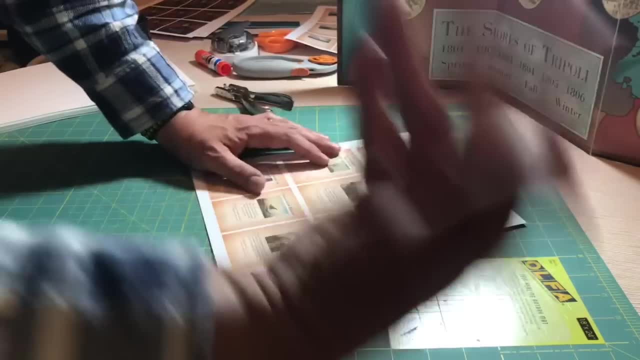 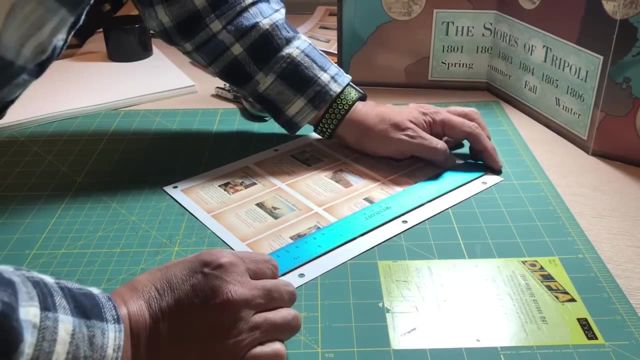 make sure that the holes are as straight as we can make them, so that the holes are as straight as we can make them. go ahead and cut these cards out, and you know what? i'm just going to leave it rolling and i'll show you how i do that. so, first of all, i'm going to cut these sides over here, i'm going to align my 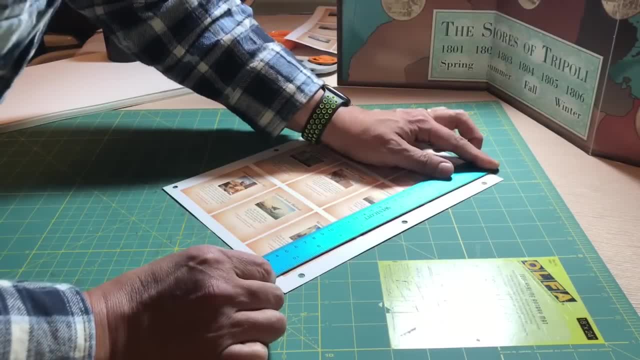 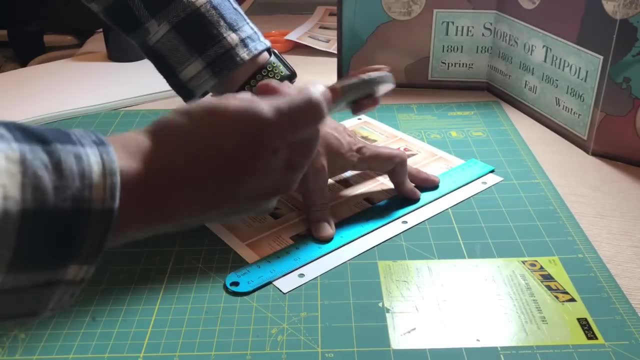 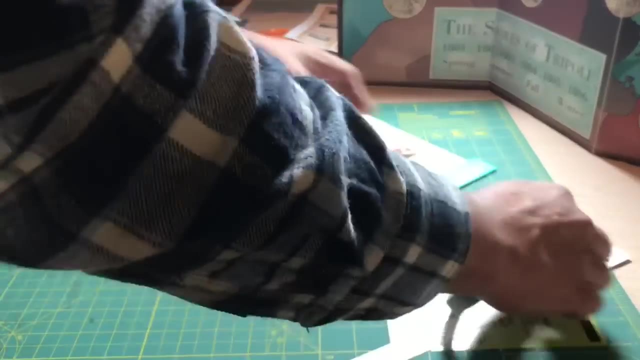 ruler. i really hope that you guys can see what i'm doing, okay, and i'm going to take my rotary cutter and hold down my ruler so that it doesn't move, and i'm going to make a few passes with my rotary cutter here. so that is one side cut. 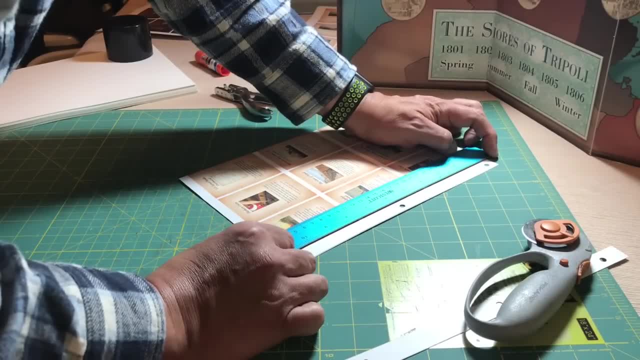 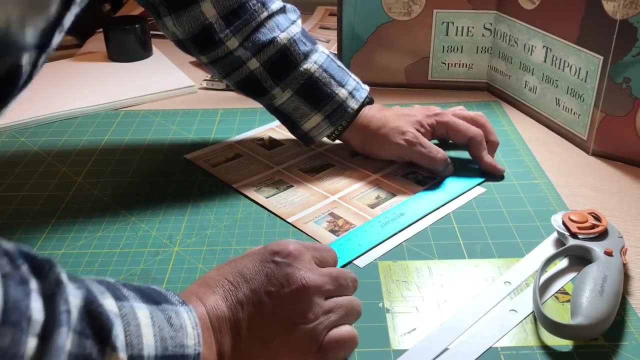 here is another side of the paper cut. so what i'm doing is cutting off the white space at the edges of the paper. you might be asking: aren't you afraid of getting hurt marking? how did you acquire the confidence to be able to use this tool? 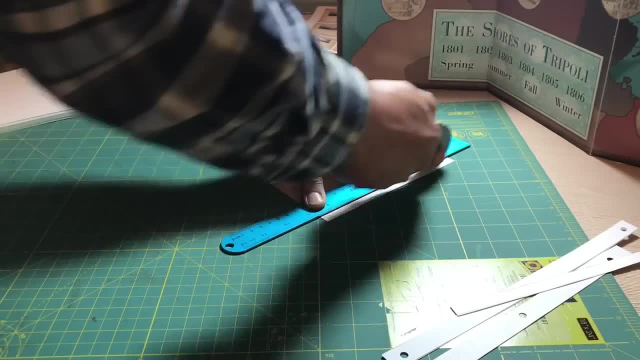 well, it took me a long time. initially, i really wasn't comfortable using a rotary cutter, and so i was using scissors or a paper trimmer or a guillotine cutter, and that was what was in my comfort zone for many, many months, until i finally just got practice enough and i just 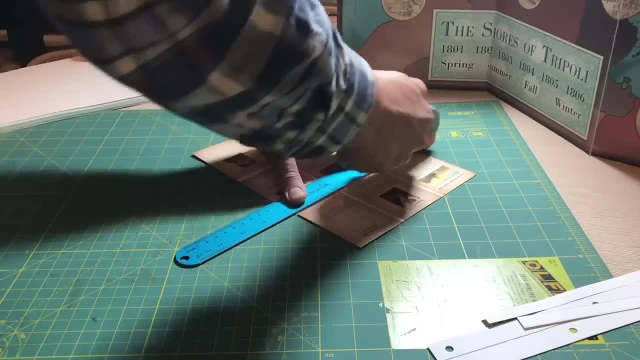 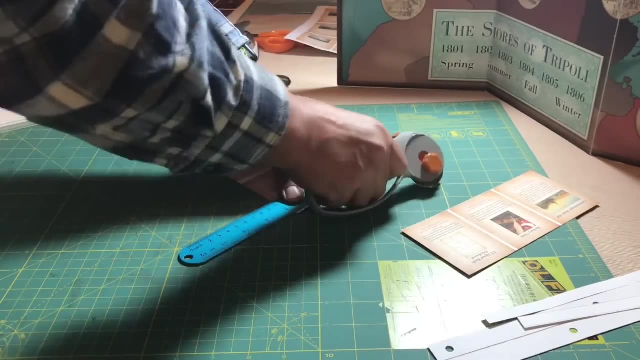 kept on pushing myself to practice using the rotary cutter because i kept hearing other people say that it is really the best way to cut, And so I just kind of basically made a concerted effort to teach myself how to use and practice using a rotary cutter, and I've gotten to the point. 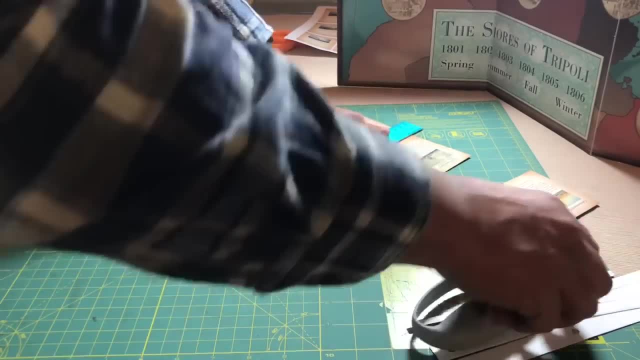 where I feel fairly confident with it, and I'm committed to using a rotary cutter to cut pretty much everything in my build. now I don't ever feel the need to use something else or maybe go back to a paper trimmer. In fact, I just recently moved my paper trimmers out of my workshop. 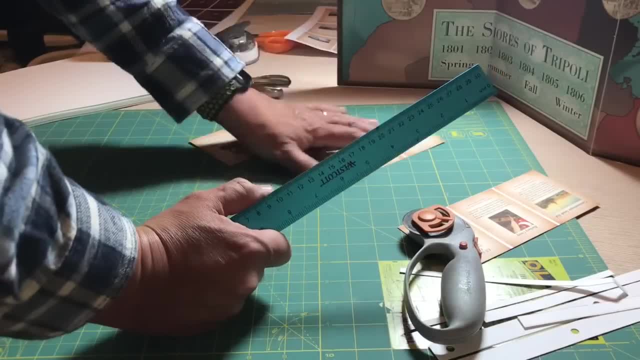 because I never use them anymore. I'm so committed and comfortable. now to the rotary cutter. Okay, let's see, Am I happy with my edges here? This one, there's just a little bit of white space. I'm going to go ahead and make. 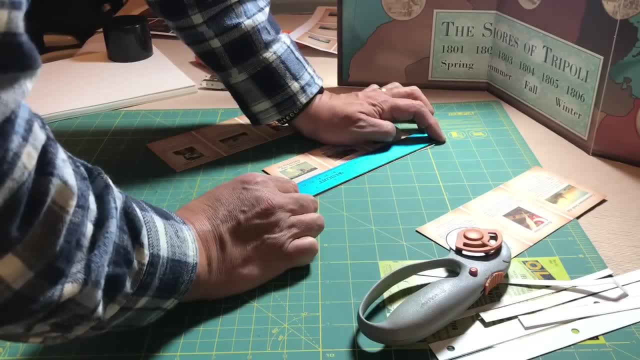 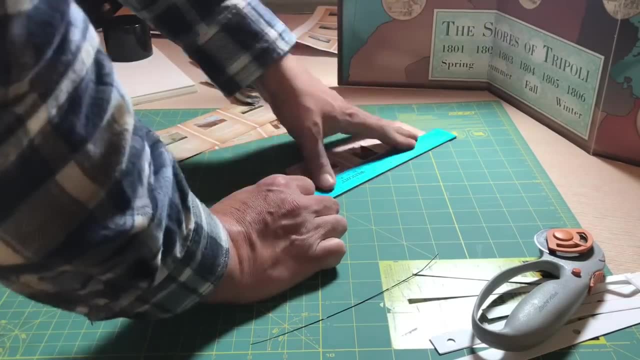 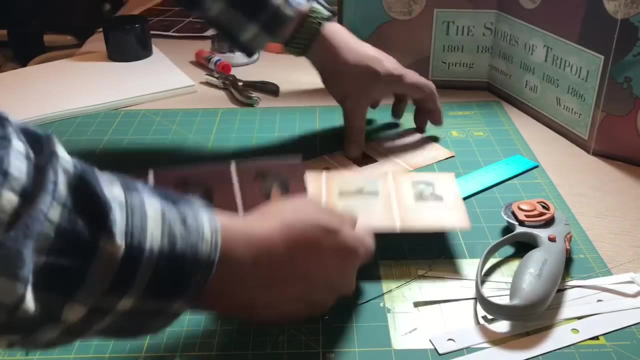 another pass there. Okay, one more pass over here. Alright, we are nearly done. This is where we are right now. We have card fronts and backs, and they're not 100% cut yet, so what I'm going to do is I'm going to lay them on top of the other. 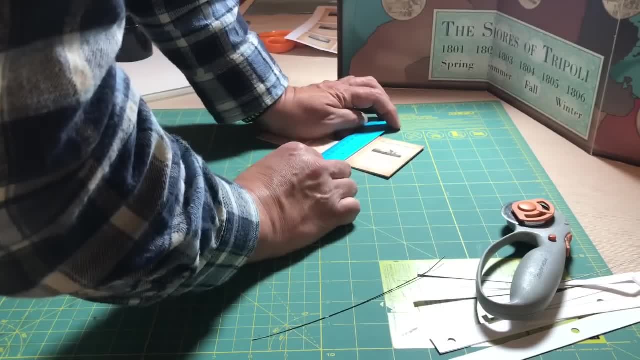 like. so make sure that they're aligned, and then I'm going to cut these down into individual cards, three layers at a time. Now you have to be careful for this one, and you have to really push down on your ruler, because the layers on the bottom tend to shift. 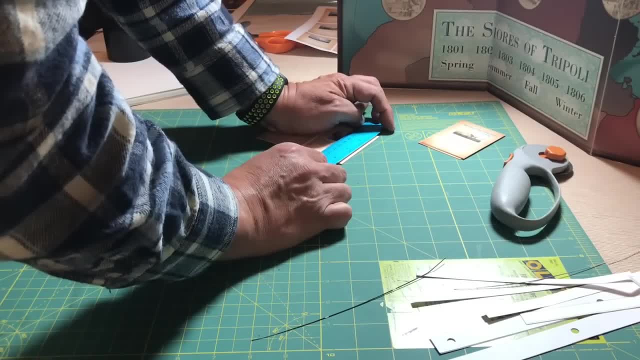 because they are not in direct contact with the court of the ruler. Now, the court of the ruler when you're holding it down, that's what makes it not shift, but the underneath layers might shift a little bit. so I tend to use quite a bit of force when I'm holding the cards down. 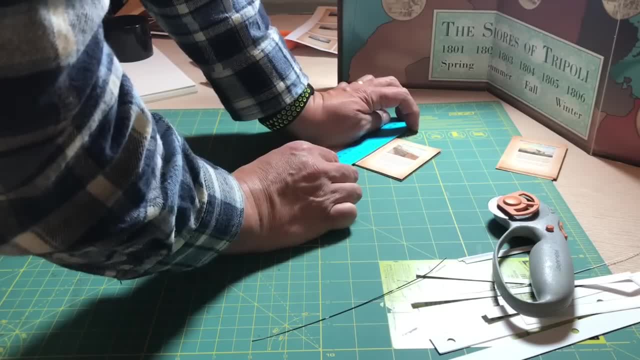 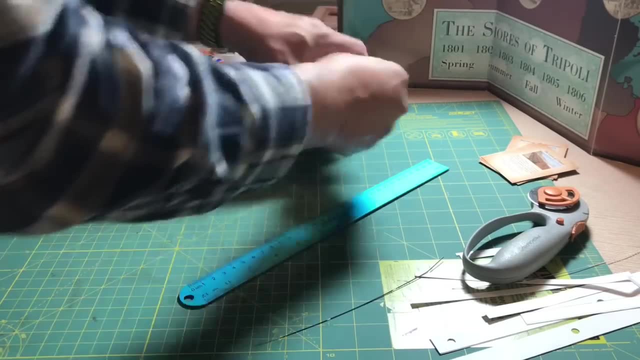 and I'm holding the ruler down. Almost done here. Alright, I'll be honest with you guys. I'm not used to talking while I'm doing this or explaining what I'm doing, so this is kind of a new experience for me. Not sure that I like it. 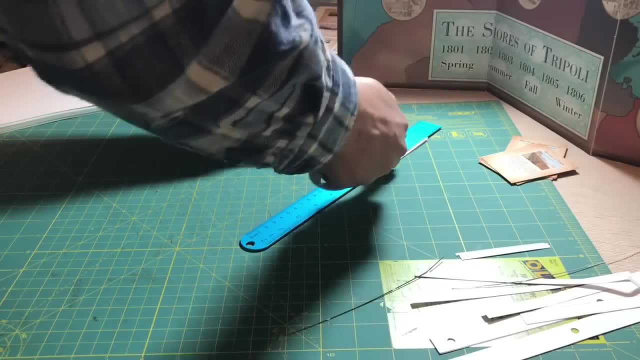 Not that I don't like explaining things or explaining things to you guys. just you know it's kind of hard for me to focus on doing two things at a time. Explain what I'm doing as I'm doing it. It makes me slightly less efficient. 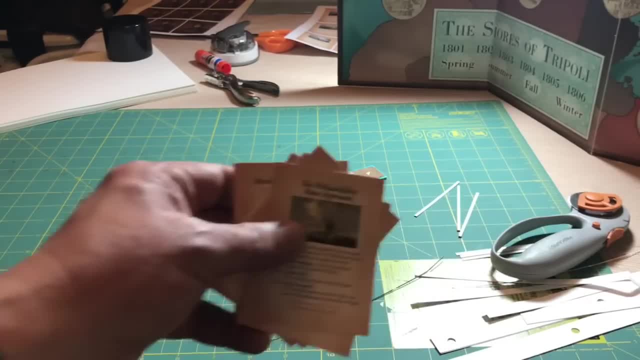 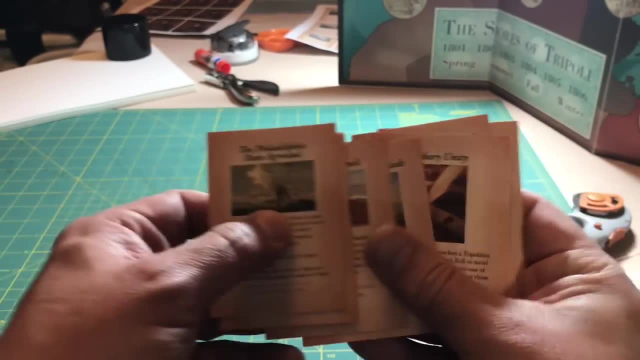 So looks like we're done, And let me go ahead and show you where we are with this. These cards are now cut and you're looking at the fronts, And so far, so good. There may be some touch-up work that I'll do. 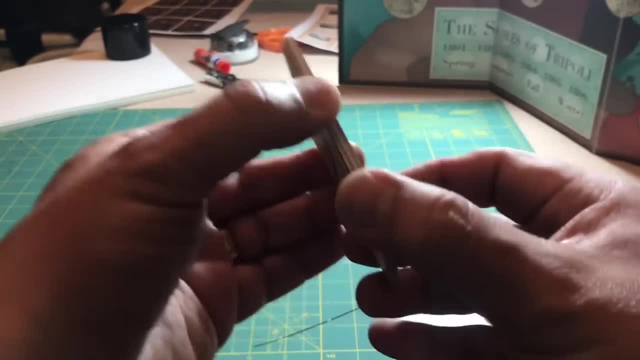 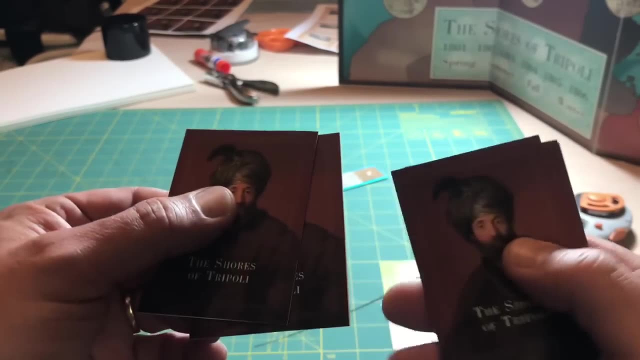 but I'm pretty happy. There's the alignment And there are the card backs. That one is a little bit, a slight bit of white peeking out. I might just go ahead and give that another pass with my card back, With my rotary cutter. 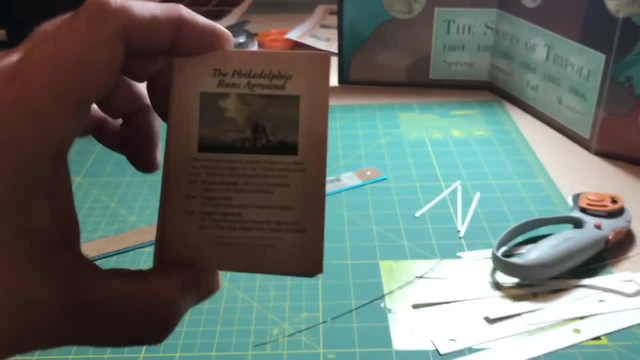 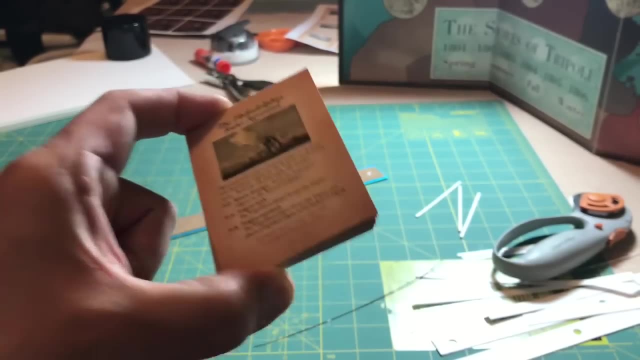 But that's essentially the process of making card fronts and backs. And now what I'm going to do, which I'm not going to bother you with on camera, is I'm just going to repeat what I just did for all of the other sheets. 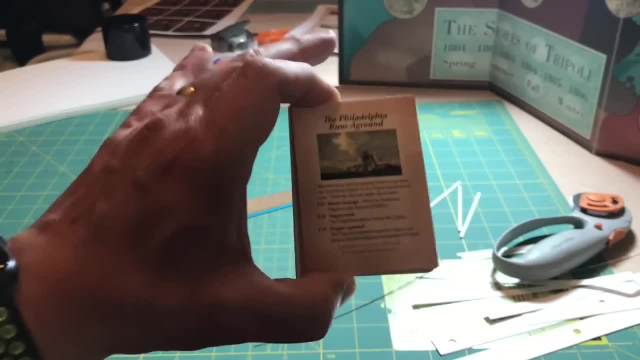 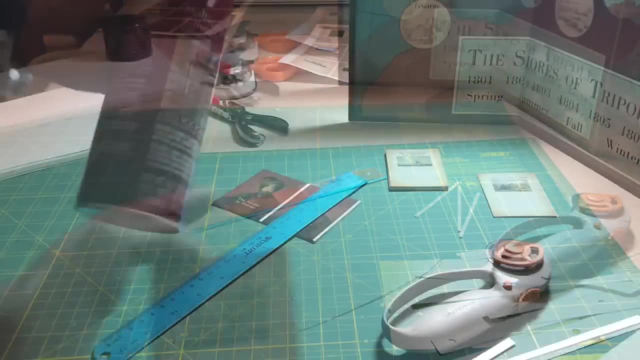 until we have the entire two decks- the US deck and the Tripolitan deck- cut out, And then we'll show you the rest of the build. I forgot to give you guys a quick reminder, Very important reminder: Do not spray your spray glue. 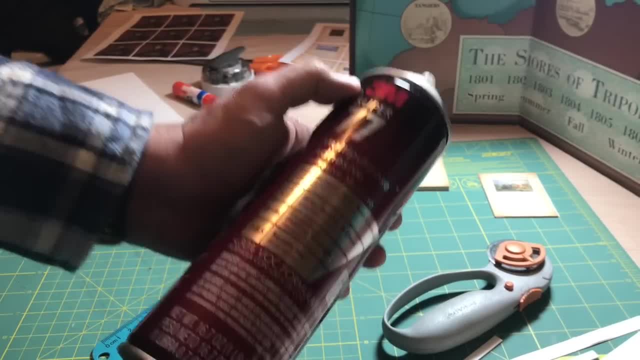 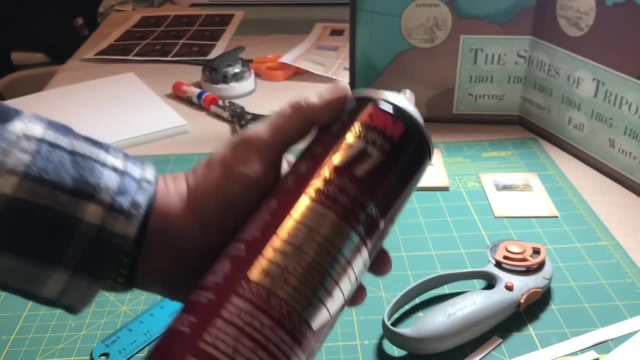 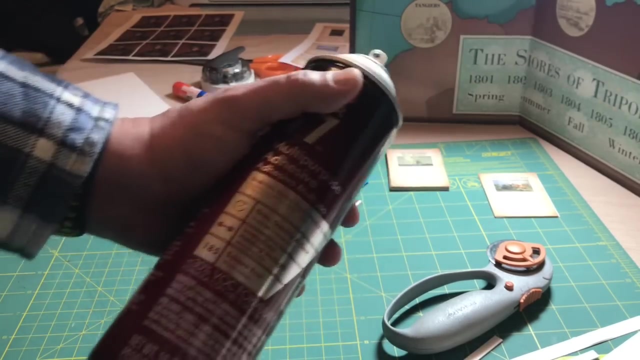 inside the house. It's going to cause property damage and stink up the place, and your significant others are going to be very, very unhappy with you. Take your spray glue and spray it outside your house. Very, very important piece You know. just wanted to give you that. 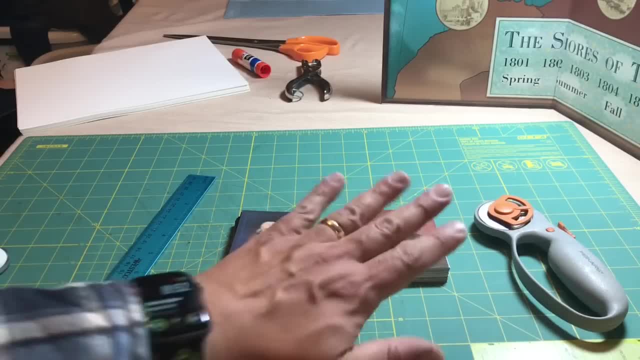 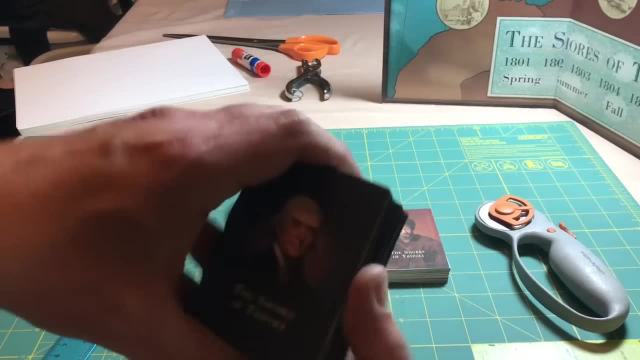 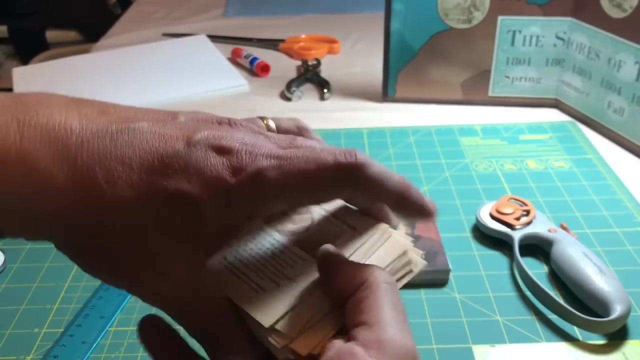 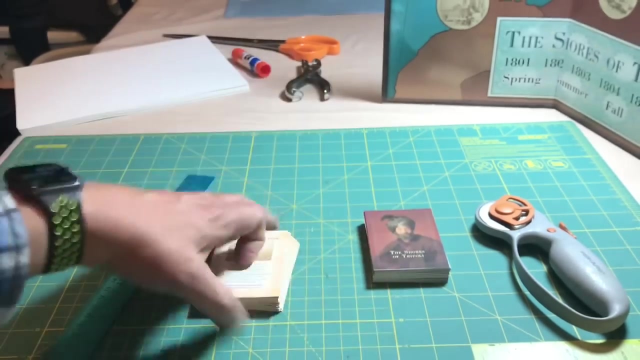 reminder Right Here's where we are now. We have completed cutting down our 56 cards- Seven of the US cards over here, And here are the card backs And here are the card fronts. I'm feeling pretty good about that. 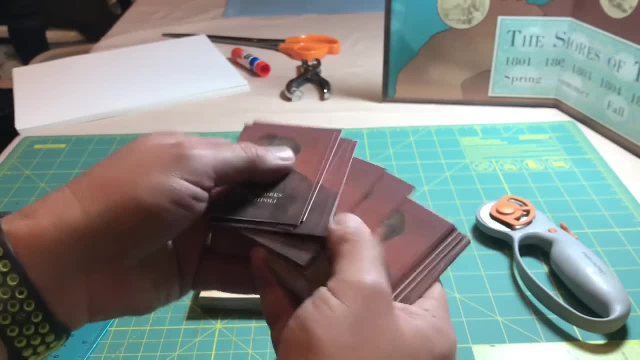 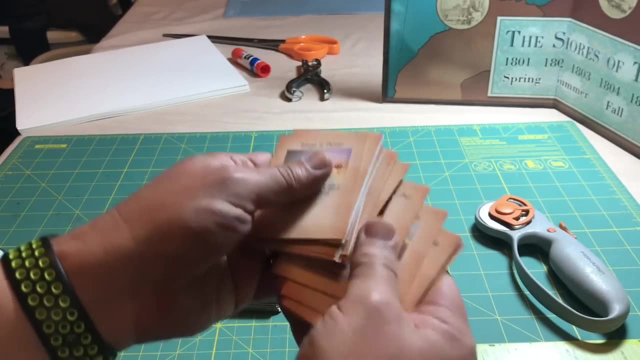 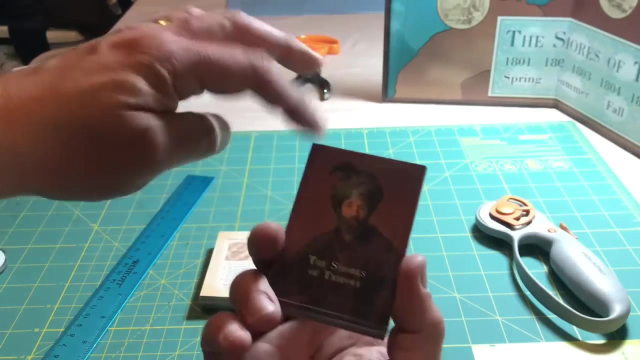 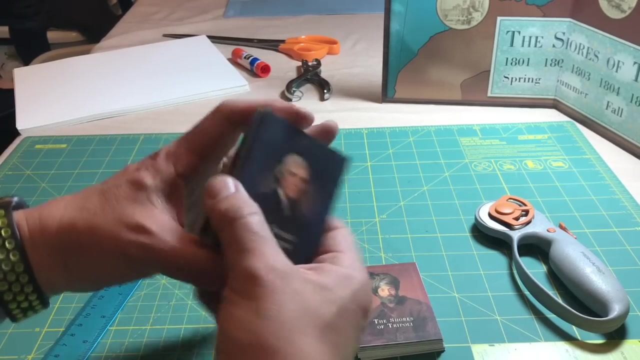 And here the Tripolitan cards: Front, backs and fronts. Okay, So we could leave these cards like this. I mean, there's nothing wrong with that And, by the way, these are roughly poker-sized cards: two and a half inches by three and a half inches, US poker-sized cards. But for me and for 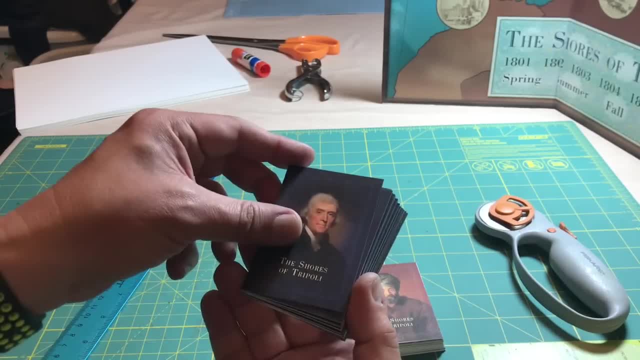 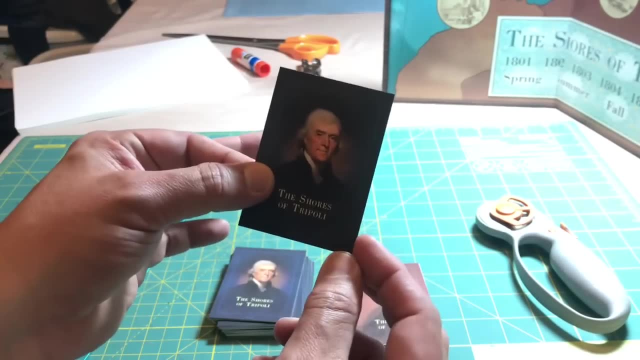 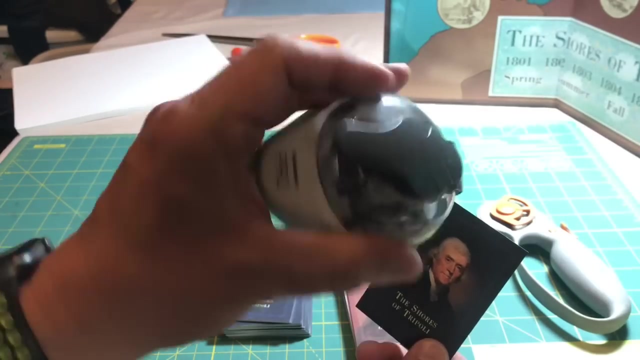 many print and play enthusiasts. there's still another step to take here, and that is to round the card corners so that we get a more pleasing and more professional look, And to do that we're going to use our Kadomaru Pro Corner Rounder. Now, the Kadomaru Pro Corner Rounder has 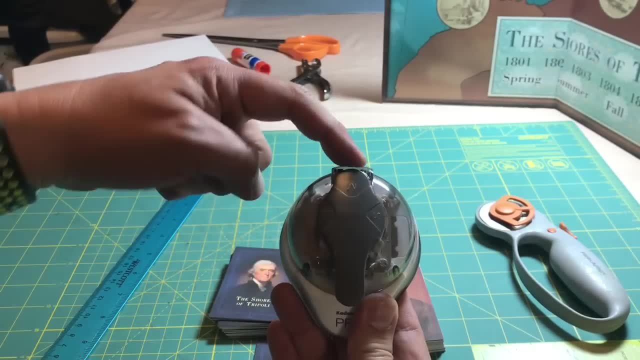 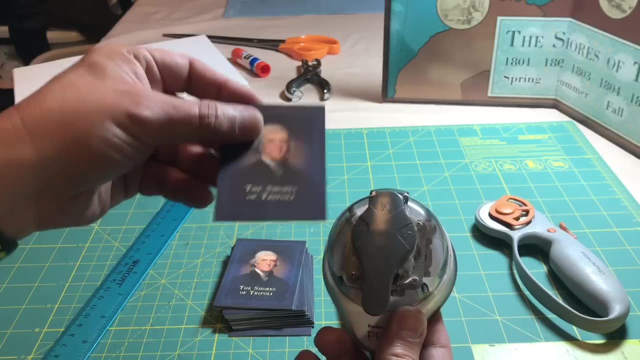 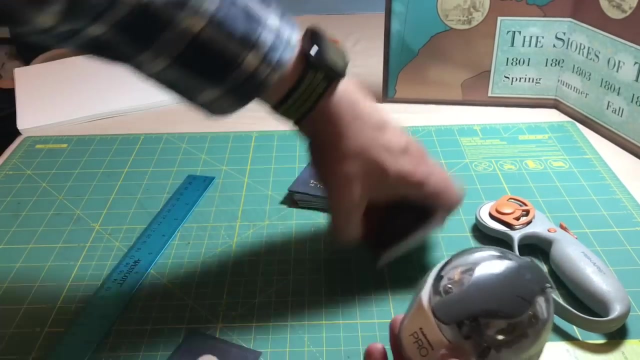 three settings: the large corner radius, medium corner radius and the small corner radius. Now for a poker-sized card like this. generally, I have come to like the small corner radius, So that's what I'm going to do right this second. So we're going to go ahead and 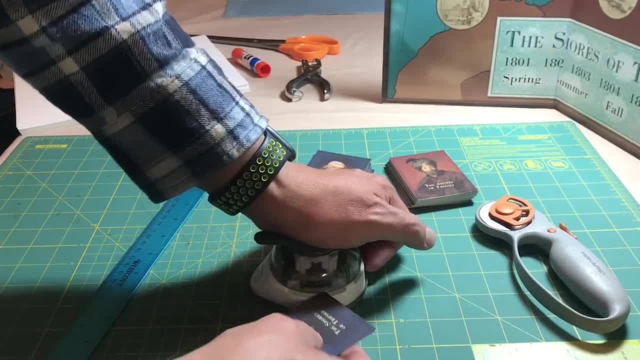 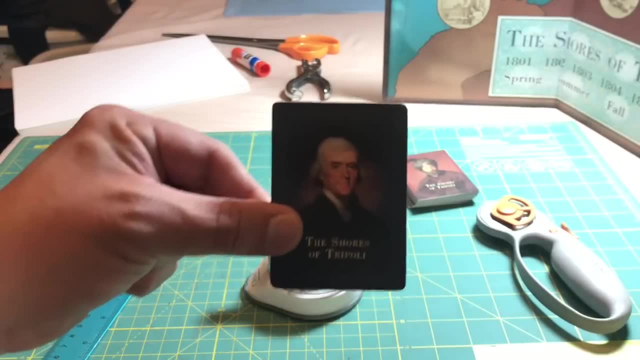 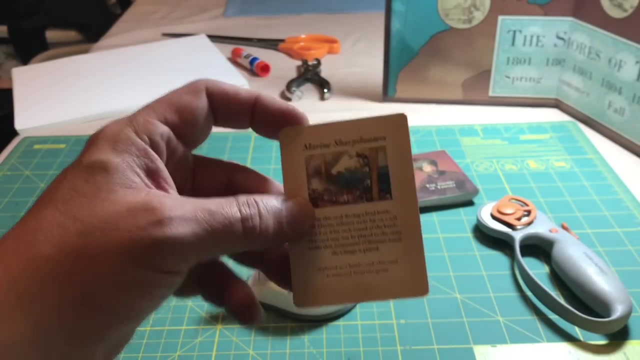 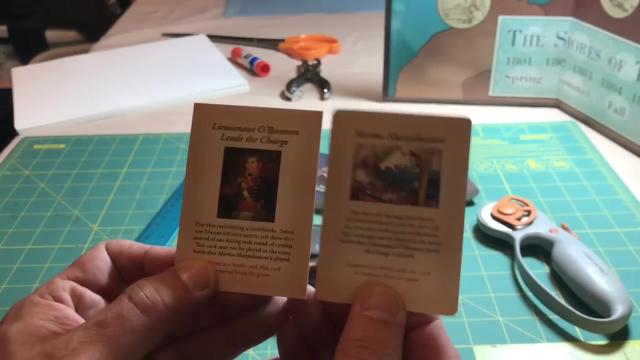 round The corners OK, and it's amazing to me what such a small little step can have a big difference in how your card looks and kind of like the feeling it gives you. Those, if you compare to the square corners here, the rounded corners, even though they're so small in radius, to me, really make a 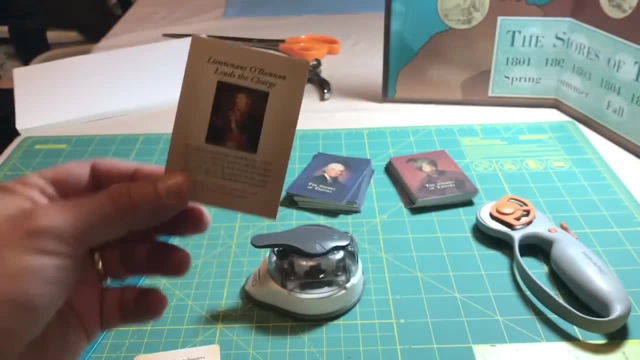 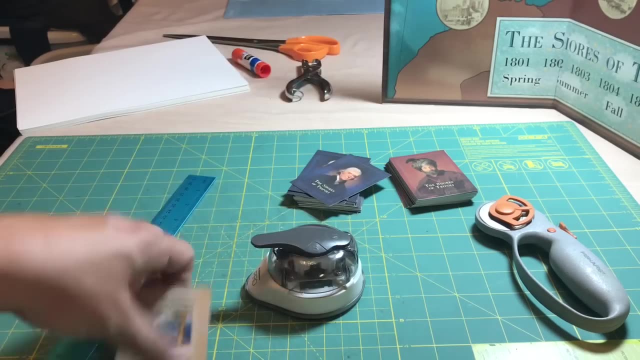 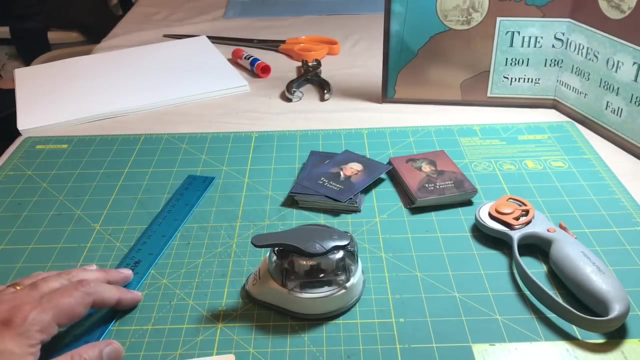 big difference, Right, OK, so we're just going to keep going. Keep on doing that for all of those other cards. So what is that? 56 times four corners to be rounded, And from my own experience, it's probably going to take me less than 10 minutes to round all. 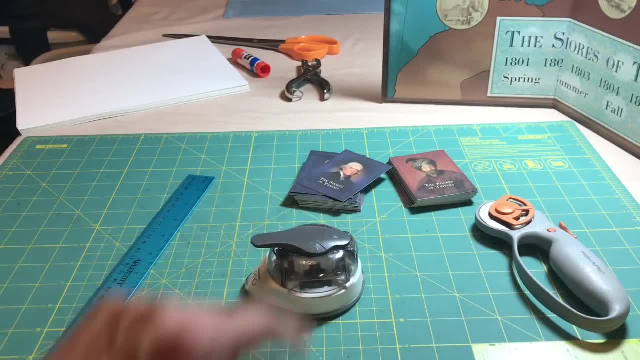 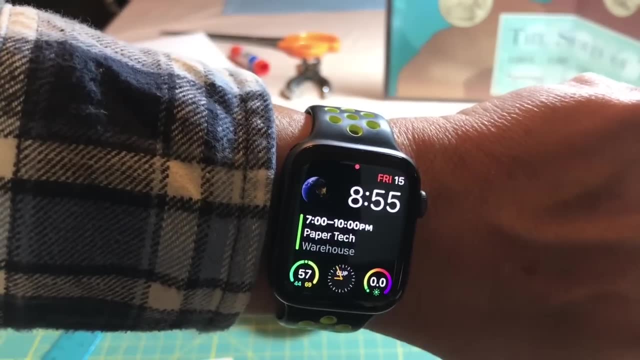 of those. I won't bore you with doing it on camera, So we'll check back in once. I've rounded all the corners Roughly about 10 minutes. So what is that? It is now five minutes to eight. Let's check back. 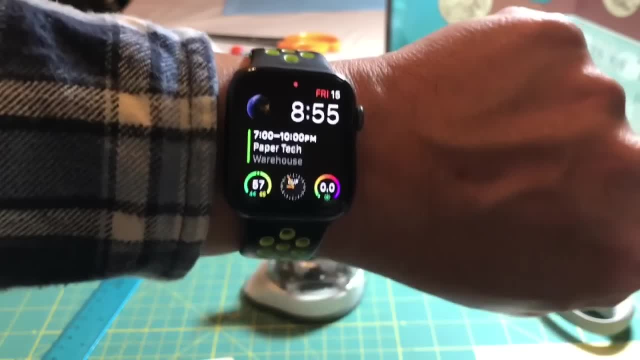 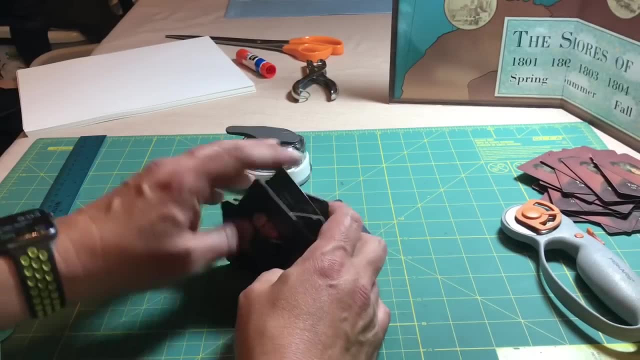 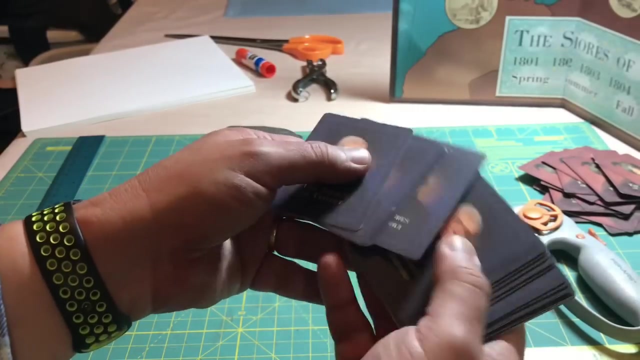 in. My goal is to be done by 9.05.. Let's, let's give myself that challenge. OK, All right. What did we say? Done by 9.05.. It is 9.03.. So in about eight minutes, I was able to round 56 times four card corners. So what is that? 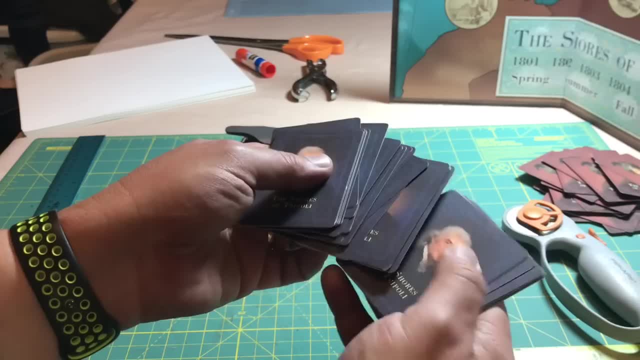 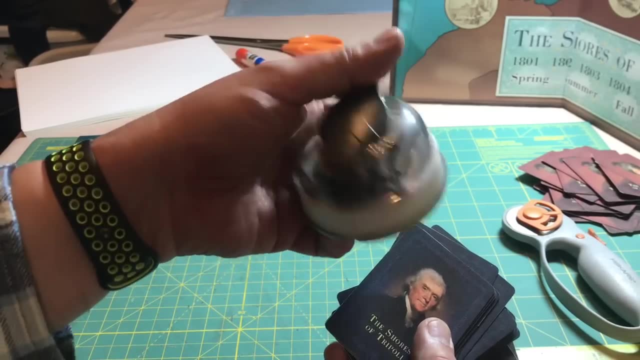 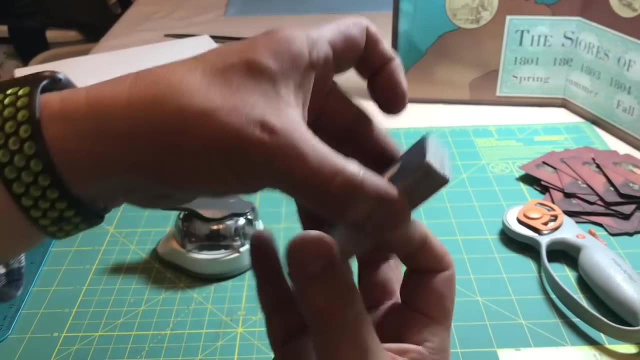 Somebody good at math. That's what? 224 corners rounded with my trusty Kadomaru Pro, And I've had this guy for nearly a year and it still keeps on going- Best ten dollars I ever Spent. So that's the US deck, with the corners nicely rounded, And let's just take a quick look. 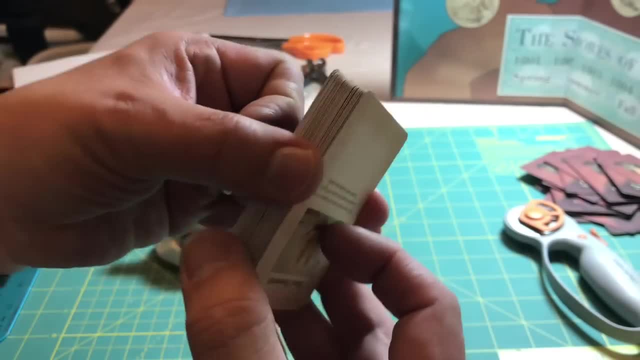 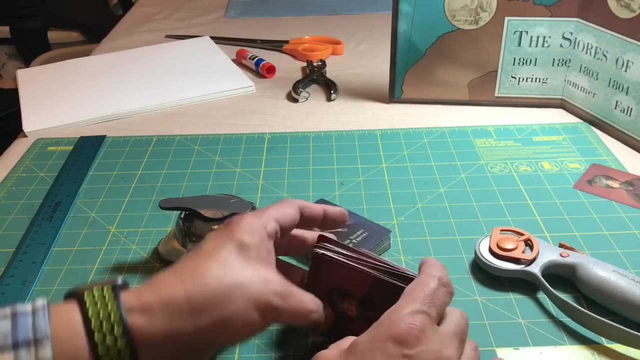 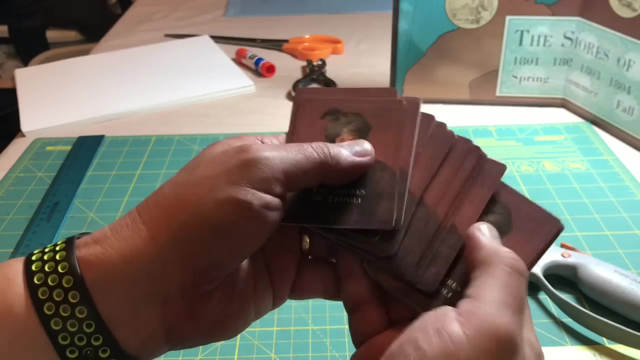 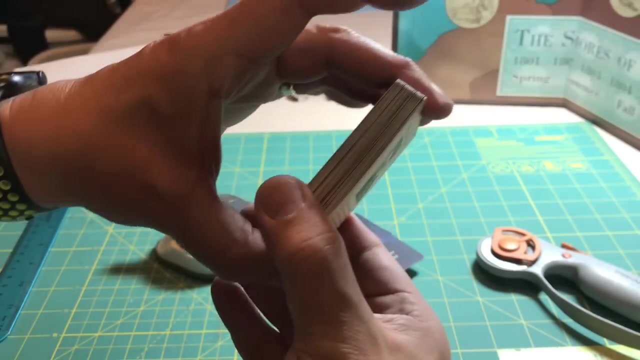 at the card alignment there. Yep, Looks pretty good. And here is the Tripolitan deck, with the corners all rounded as well, Mm, hmm. And the deck Alignment, Considering that this was all done manually with rotary cutter and with cork back. 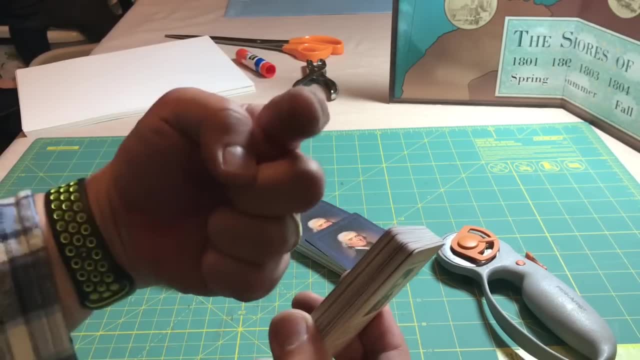 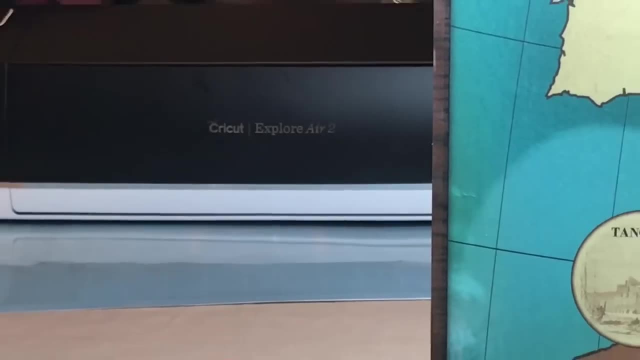 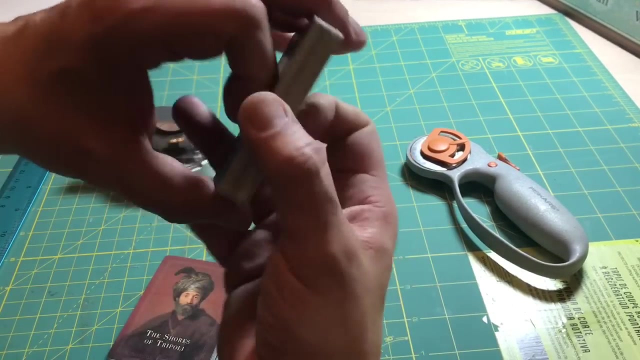 ruler and with my eyes pointing at my eyes and and not with that machine over there, not with that cricket that I have over there which I sometimes use to cut things. So sometimes I like to do things manually, Sometimes I also like to experiment with a cutting machine, But we're 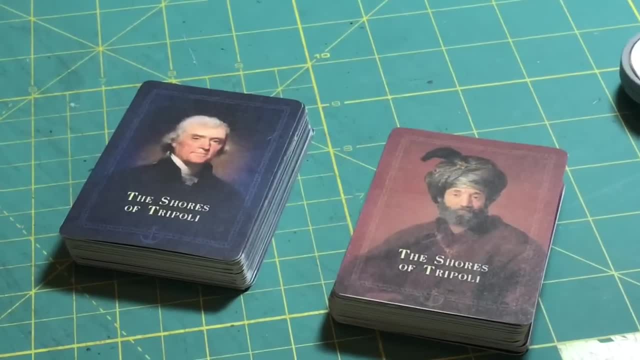 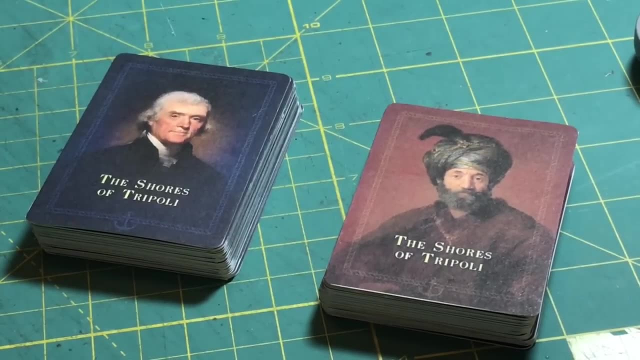 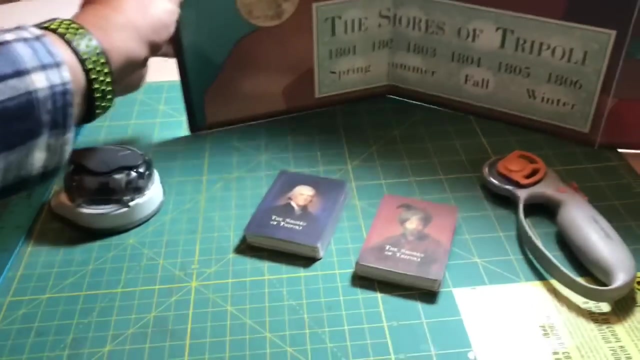 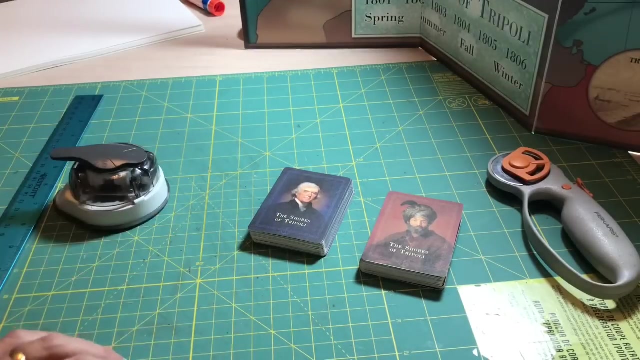 essentially, essentially pretty much done with these 56 decks of cards, these 27 cards per deck for this game, Zooming out here The Shores of Tripoli. Once again, a war game, a small box war game, war game that is still under development, is still under beta testing by a gentleman named. 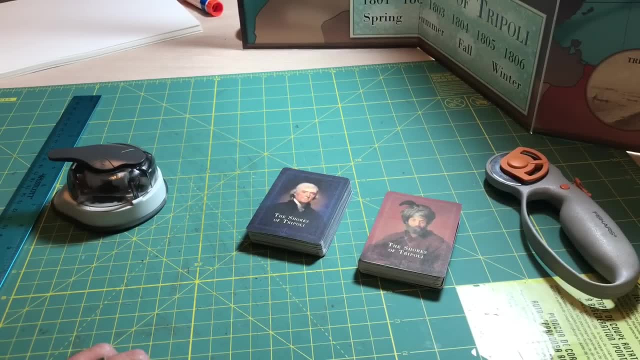 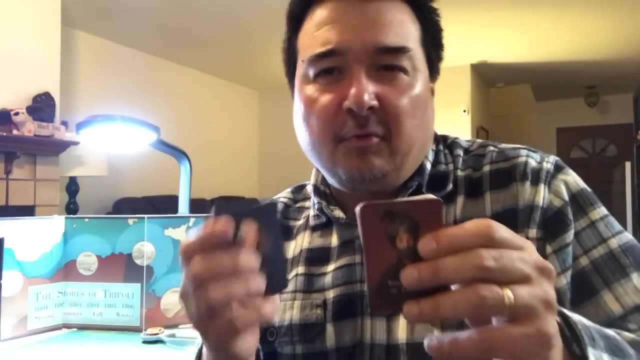 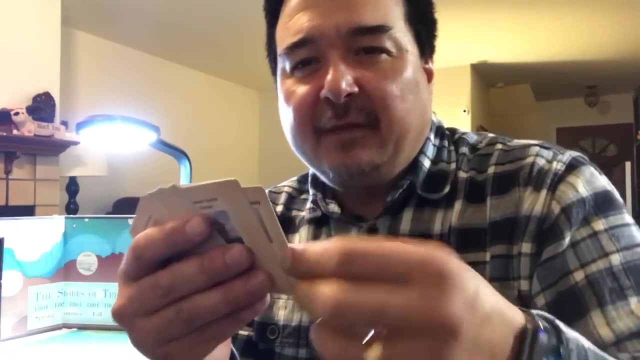 Kevin Bertram. Let me just pause For now. Well, there you have it. I completed making a deck of cards and I hope that I was able to share with you my usual process. just to review each one of these cards is three layers layer of plain paper. 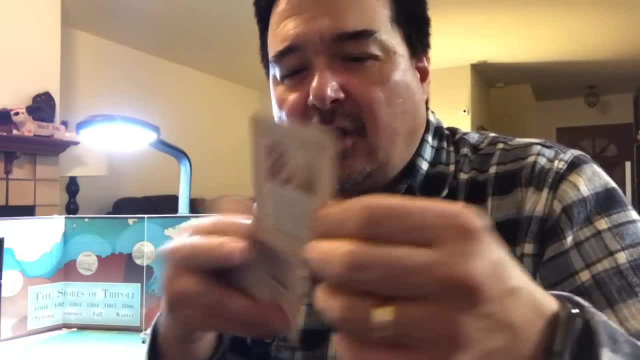 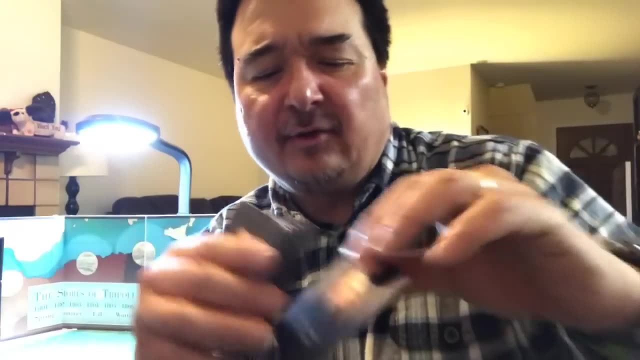 on the back, layer of plain paper, on the front with a layer of card stock sandwiched in between, And that gives us cards that look like this: Now, these cards don't riffle shuffle and I wouldn't try to riffle shuffle them because, unlike what they make actual cards out of.